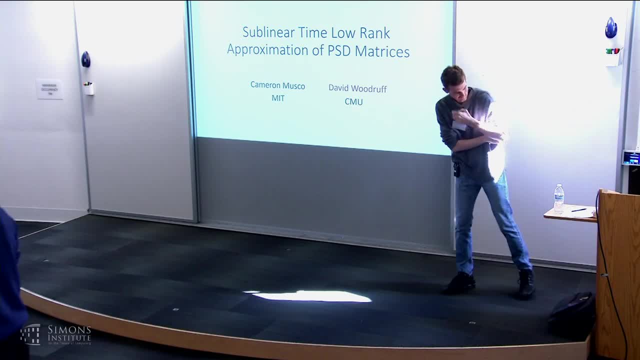 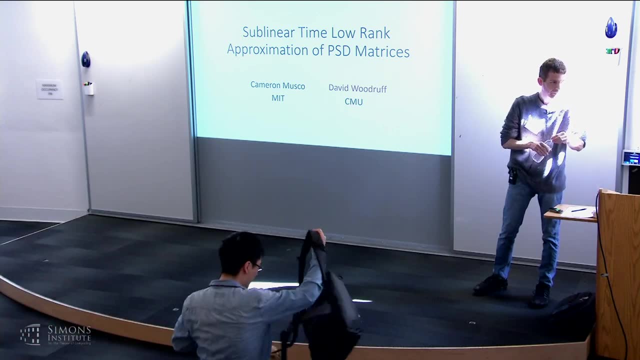 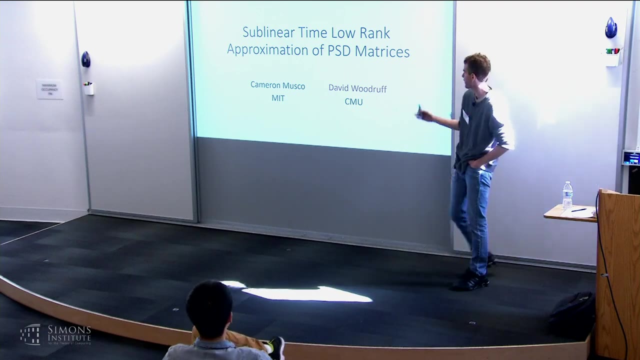 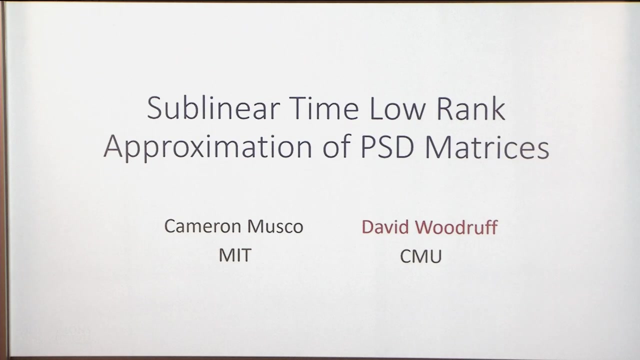 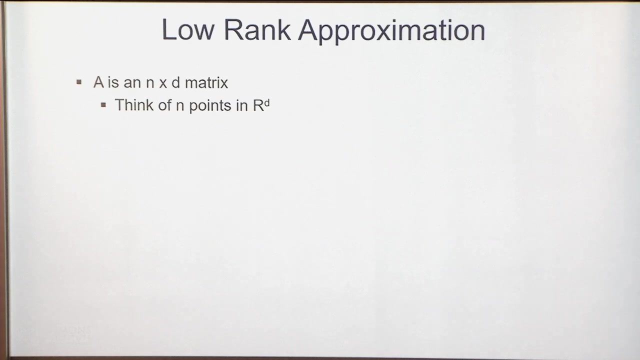 So thanks to the organizers for inviting me. This was done when I was still at IBM Almaden with my intern at the time, Cameron Musco, So sublinear time. low-rank approximation of positive semi-definite matrices is the title. Let me first define the low-rank approximation problem. 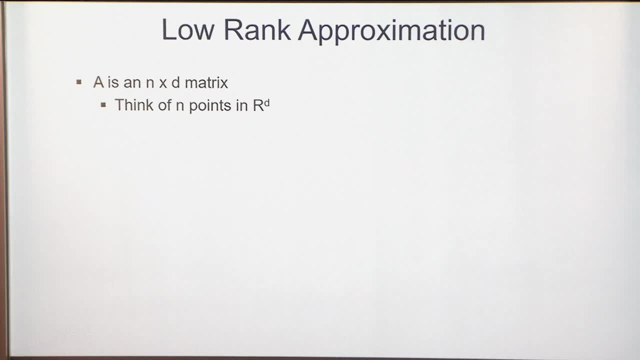 So we're given an N by D matrix A. Think of the N rows of A as being points in R to the D. For example, A might be a customer product matrix Aij indicates how many times customer I purchased some item j. 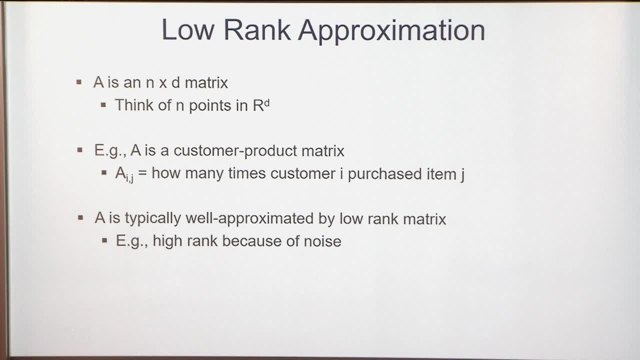 In many applications A is well approximated by a low-rank matrix. There might be some underlying latent variable model or whatever, but typically A is well approximated by a low-rank matrix. The goal is just to find a low-rank matrix approximating A. 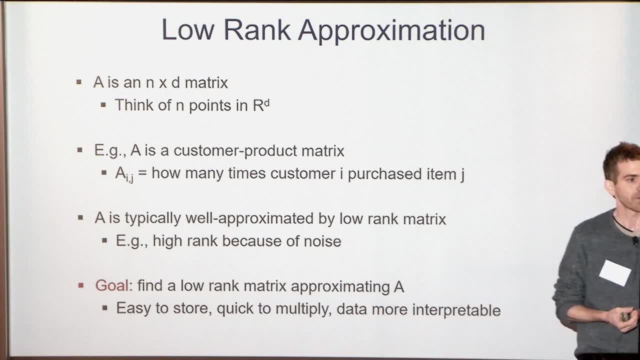 So a low-rank matrix is easy to store in factored form. It has many fewer parameters If it's an N by K and times a K by D matrix, I only have N plus D times K parameters. It's quick to multiply by a low-rank matrix because I can. 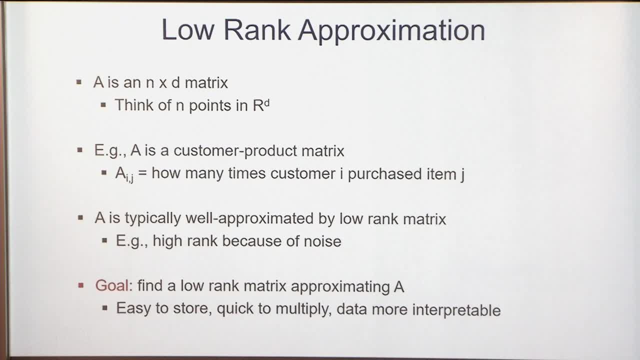 multiply a vector, first by the first low-rank factor, then by the second low-rank factor and really, if A is only high-rank because of noise, you can think of this low-rank factorization as denoising your data. 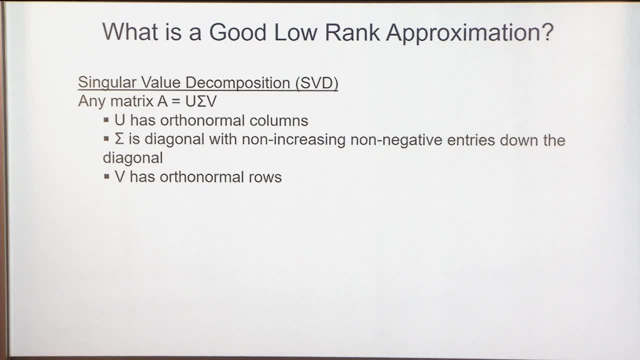 So what is a good low-rank approximation? The standard way of getting a low-rank approximation is through the singular value decomposition or SVD. So recall that any matrix A can be written as U, Sigma V, where U has orthonormal columns. 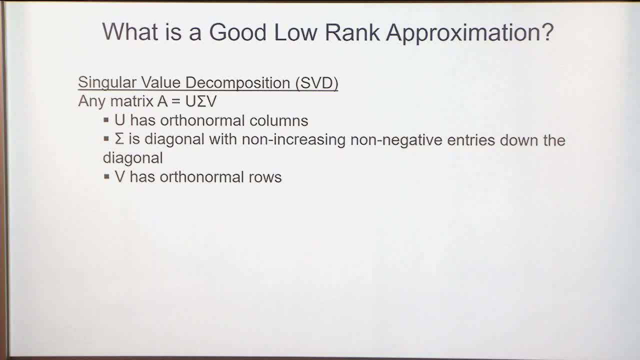 Sigma is a diagonal matrix with non-increasing entries as you go down the diagonal non-negative, and V is orthonormal rows. The standard way of getting a low-rank approximation is via the truncated SVD. So what you do is you just take Sigma. 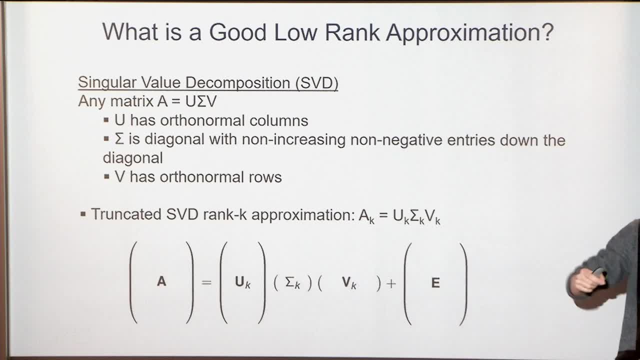 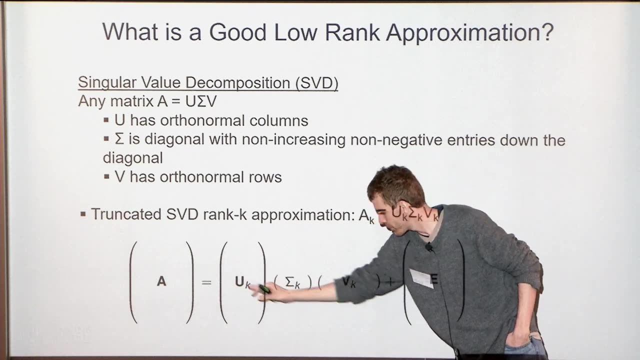 they're decreasing as you go down the diagonal. So you just take the top K singular values, the diagonal entries of Sigma, leave them alone and zero out all the remaining singular values. This gives me Sigma sub K and this effectively selects the K leftmost vectors in U. 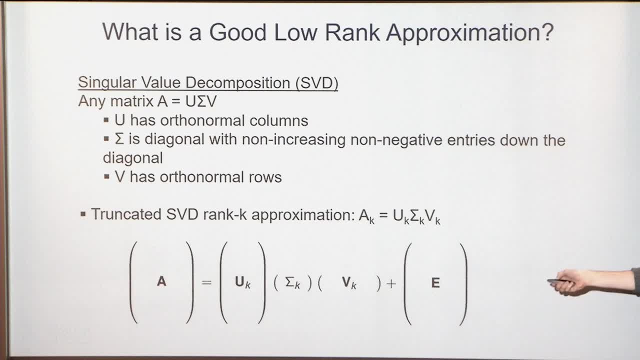 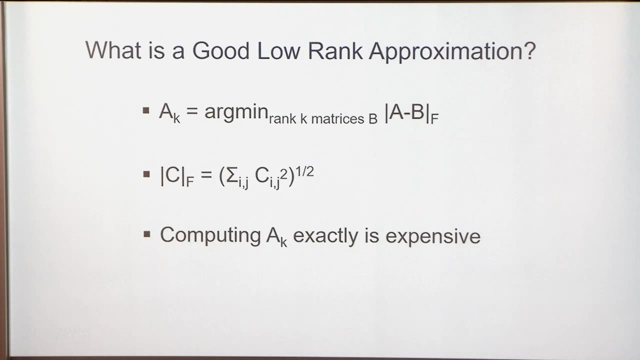 and the K uppermost vectors in V. This gives me a rank K matrix which I'm calling A sub K. So this approximates A up to some error. matrix E, which depends on all the remaining singular values. Okay, So why do people use the truncated SVD for low-rank approximation? 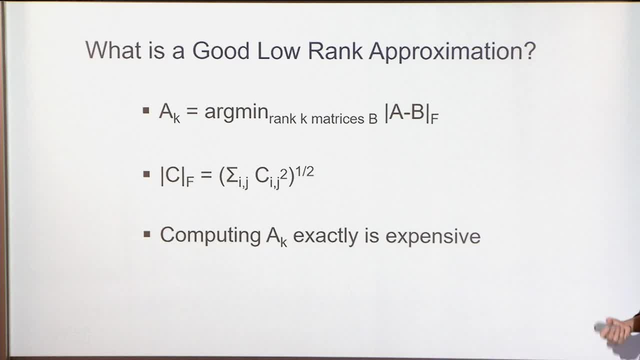 Well, A sub K is the best rank K approximation for A under a variety of different norms. in particular it's the argmin over rank K matrices B of the Frobenius norm of A minus B, where the Frobenius norm is just the sum of squares of entries to the one-half. 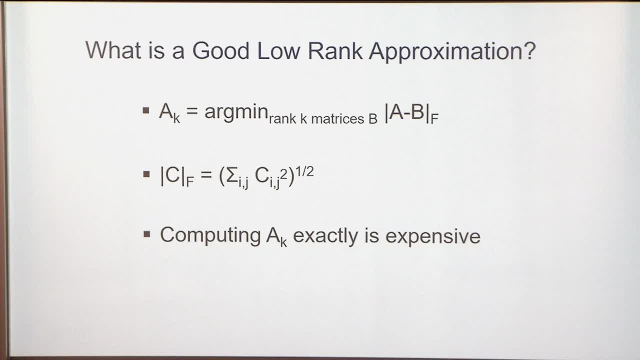 So the issue with the truncated SVD is actually that computing A sub K is expensive. Okay, So computing this exactly using the SVD can take N D squared time if A is an N by D matrix. We want to get much faster algorithms than those based. 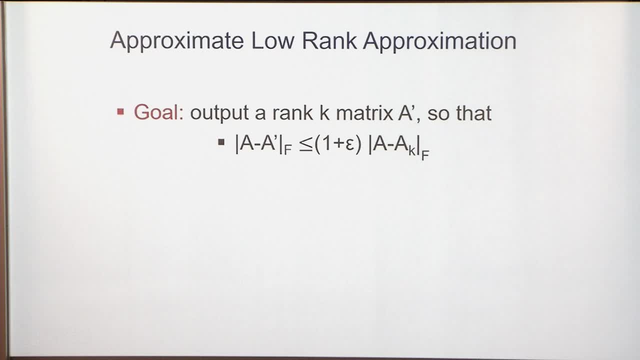 on the SVD. So people have been looking at a notion of approximation for low-rank approximation, which is a relative error notion defined as follows: So the goal is to still output a rank K matrix. let me call it A prime, so that the Frobenius norm now of A minus A prime is at most relative error. 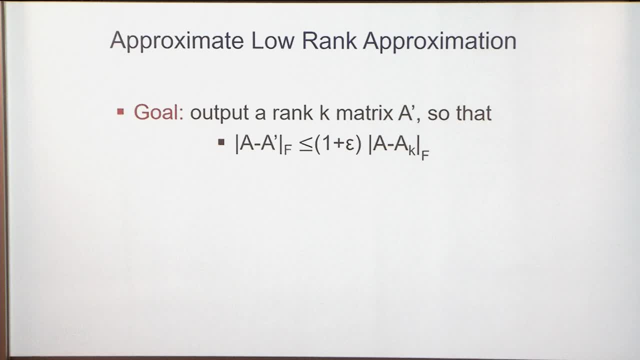 one plus epsilon times the best possible low-rank approximation cost given by the SVD. Okay, And you allow some probability of failure. With this relaxation you're able to get significantly faster algorithms, In particular in work with Ken Clarkson. 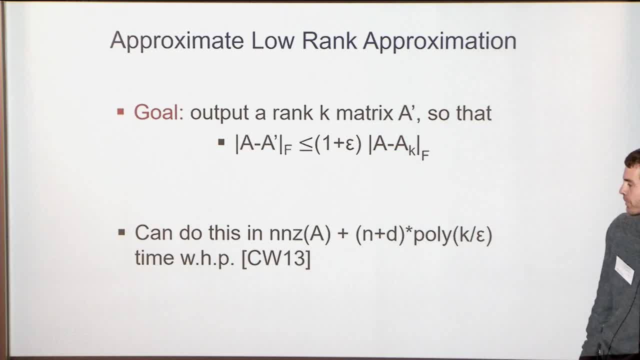 we showed that with this notion you can get an algorithm which runs in time: N and Z of A, where N and Z denotes the number of non-zero entries of your input matrix A. Okay, So this algorithm is sensitive to the sparsity of your matrix A. 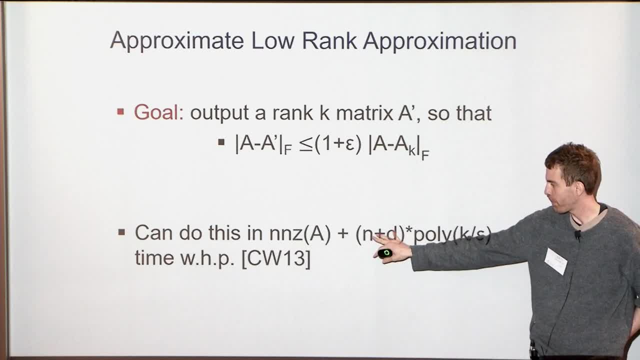 Plus what is typically a low-order term, N plus D, the sum of the two matrix dimensions times a polynomial in the rank parameter K, which is typically small, and one over epsilon for a one plus epsilon approximation. Okay, So just some perspective. 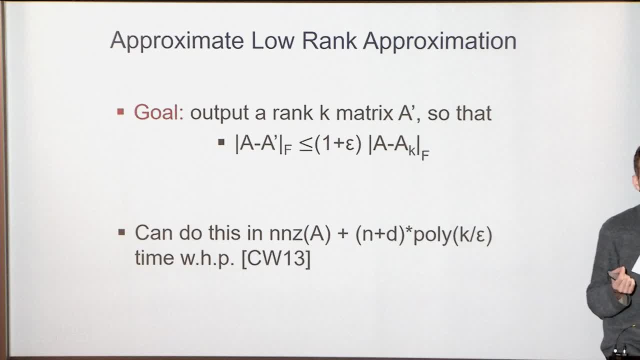 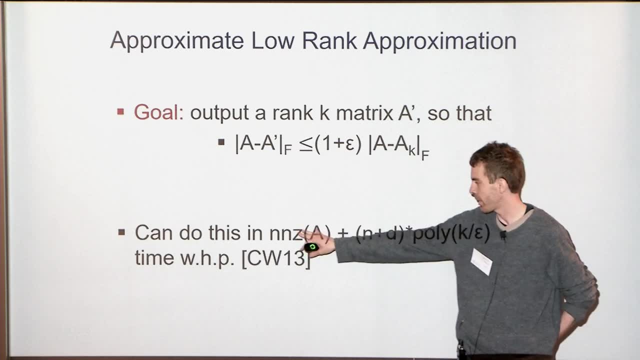 Even for dense matrices that have, say, N D entries, the SVD would take N times D squared time, whereas this algorithm runs in only N D time. And if N and Z of A is significantly less than that, like around N plus D. 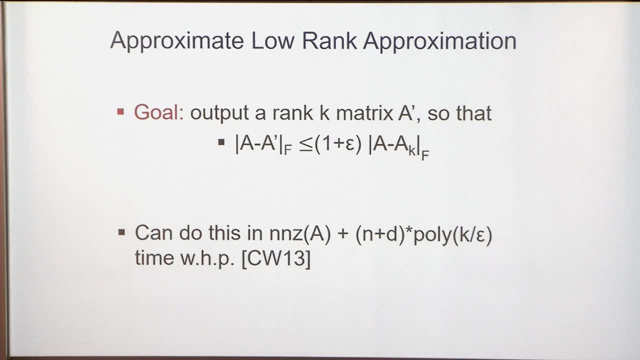 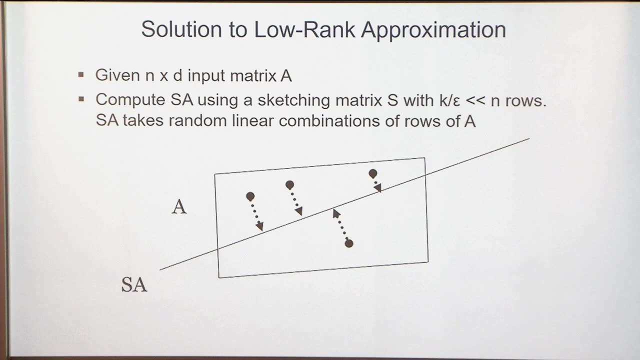 then this could be close to an N plus D time algorithm. Okay, So, and stop me at any point if there are any questions- Let me just go over roughly how you use a technique called sketching to achieve these algorithms that run in time proportional to the number of non-zero entries of A. Okay, 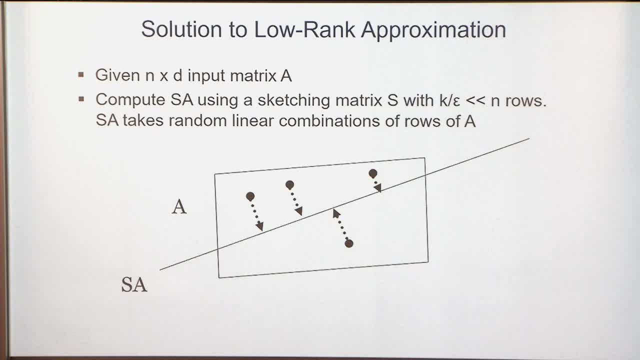 So we're given this N by D input matrix A, and we think of the rows of A as being N points here in r to the D, And the first step of these algorithms is to choose a random matrix S, And I'll discuss just a few families of matrices in a moment. 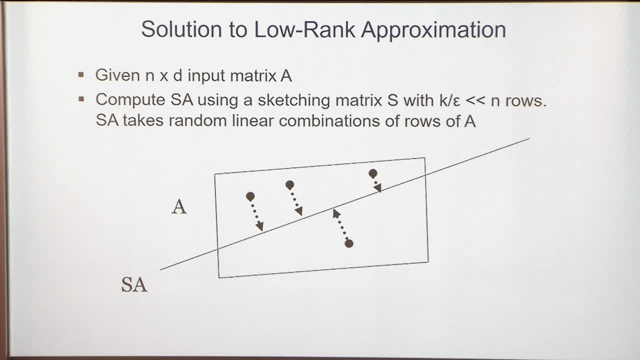 But the important property about S is that it's a very wide, fat matrix, Okay, So it has a very small number of rows, has roughly K of epsilon rows, okay, and the number of columns is n, and what we do is we compute s times a. 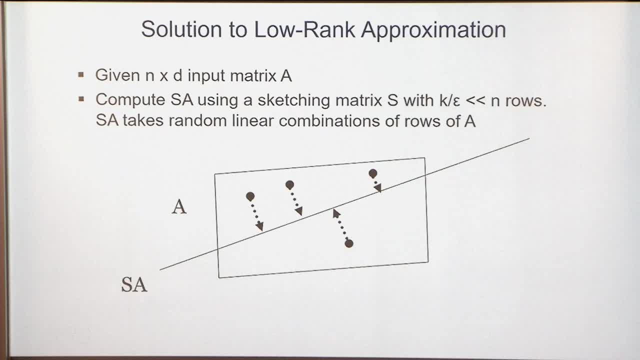 okay, this is the first step of the algorithm. now what is sa doing is taking random linear combinations of these n points, the rows of a in r to the d, and we can look at s times a. so it's a k over epsilon. by d matrix, we can think of the span of the rows of s times a. 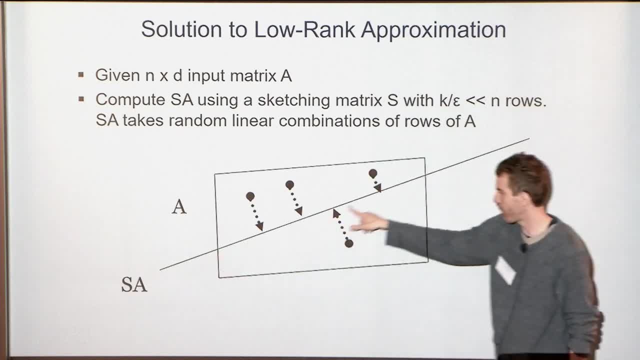 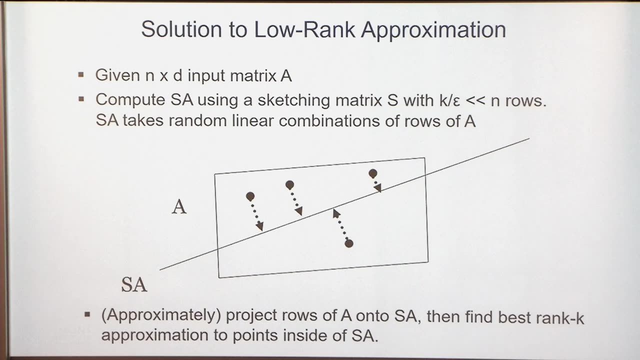 as being a k over epsilon dimensional subspace of r to the d, which i've drawn here as a line. okay, so this line represents the row span of s times a, and the next step of the algorithm, after computing s times a, is to take each of the rows of a these points and to project. 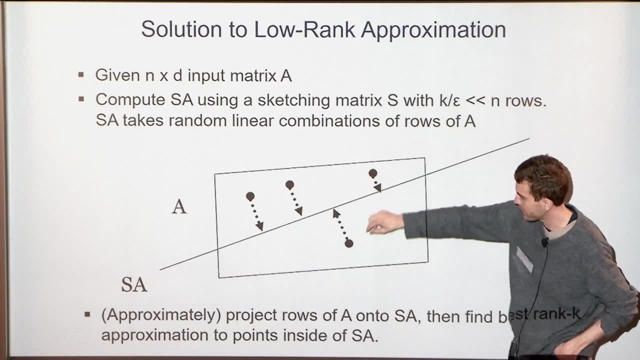 the point on to s times a. right, just move it to the closest point in s times a. okay, and now i still have n points, but they're all sitting inside the row span of s times a, which is a very low dimensional subspace of r to the d. so recall that the svd. it took number 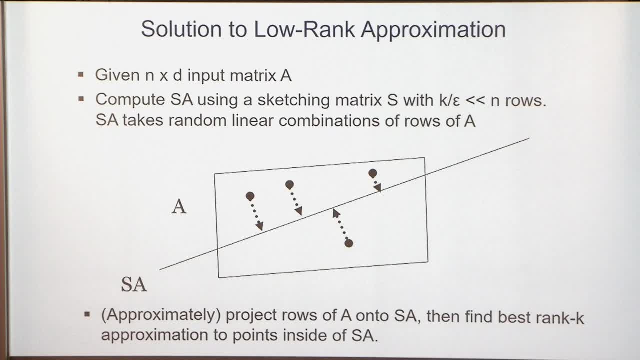 of points times dimension, squared time. now i still have n points, but the dimension of these points, since they sit in this k of epsilon dimensional subspace is, oh you know, is only k of epsilon, so i can afford to run the svd now. uh, on these projected points, if i use the coordinate, 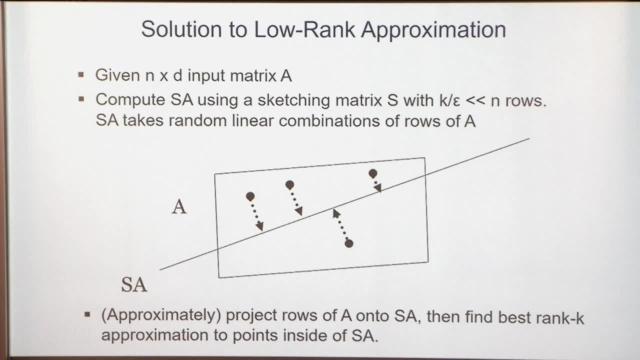 representation in this low dimensional subspace. okay, so that's uh the idea, um the uh. so one issue with this algorithm is you can't actually afford in n and z of a time to project these points exactly onto this space s times a, but uh, projection is just uh, least squares regression. 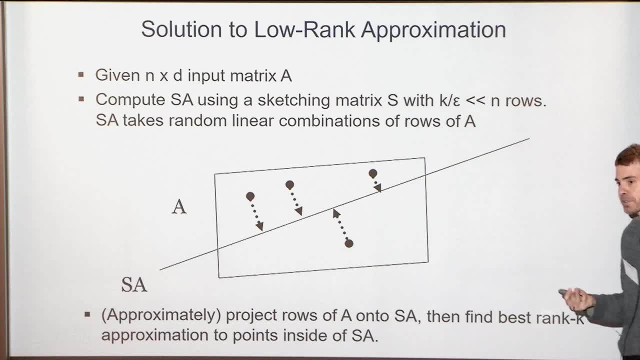 and there are many sketching algorithms, randomized algorithms for approximately doing projection. so you can approximately move these uh. you move them to an approximate closest point and the algorithm still works okay. so this is how you get um. um, this is the basic paradigm for applying sketching uh to low rank approximation, and a natural question here is: which random? 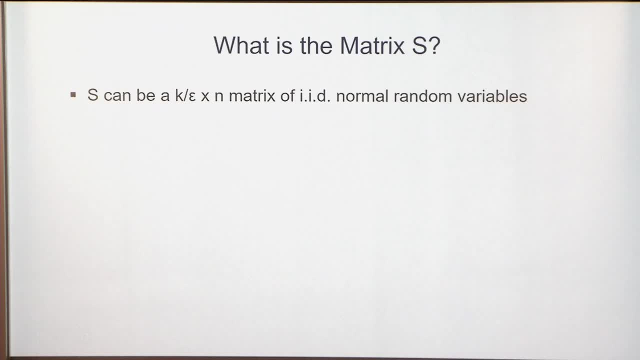 families of matrices s do you use um? so the first one that might come to mind are is a matrix of iad, normal random variables. uh, this matrix s works, but uh, computing s times a is slow because s is a dense matrix um, what sarlo showed is, instead of choosing this random family of matrices, if you choose a family, 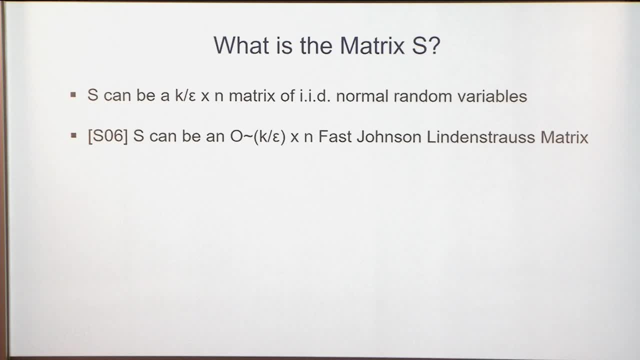 of matrices from a much more structured family called fast johnson lindensroth transforms. then you still have roughly k of epsilon rows, but now s times, a can be applied in roughly nd time, which is, uh, very fast. um, it's linear in the product of the 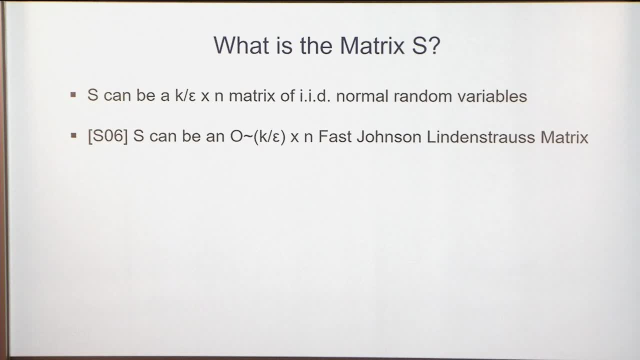 dimensions of your input matrix um. however, one drawback about this is s can't exploit sparsity in a. so if your input matrix a has a small number of non-zero entries, you could hope to do better, and what we showed in that paper with clarkson is that instead, if you choose s to be, 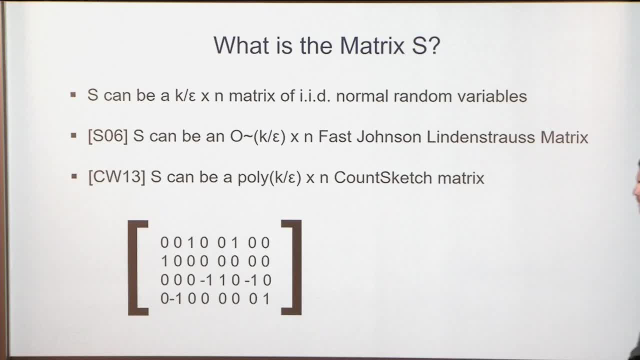 what is called a count sketch matrix. it has a bit more rows than before. instead of just k epsilon rows has roughly k-epsilon-e squared over epsilon rows roughly, but still independent of n and d and still very small. So it's still a wide, fat matrix. But a nice property about this count sketch matrix is 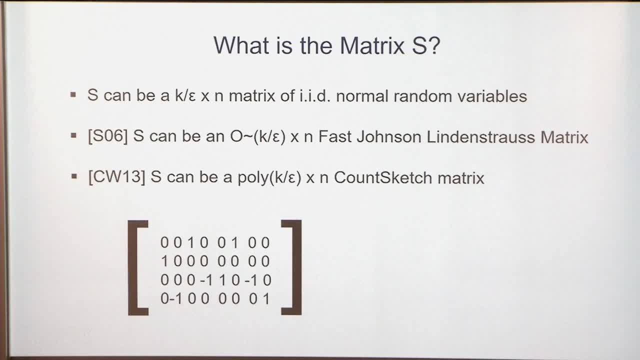 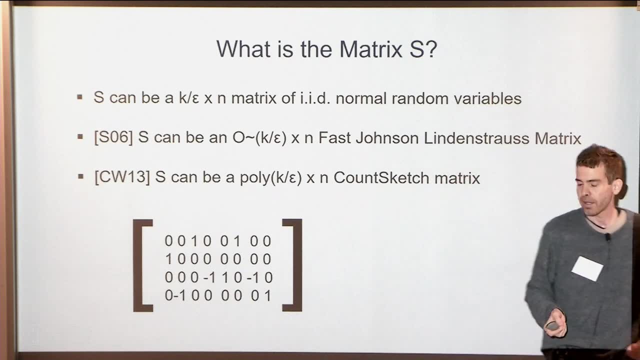 that it's extremely sparse. So each column of this matrix S only has a single non-zero entry in it. That entry is chosen at a uniformly random position in each of the n columns And that position is set to be 1 with probability 1 half, and minus 1 with probability 1 half. 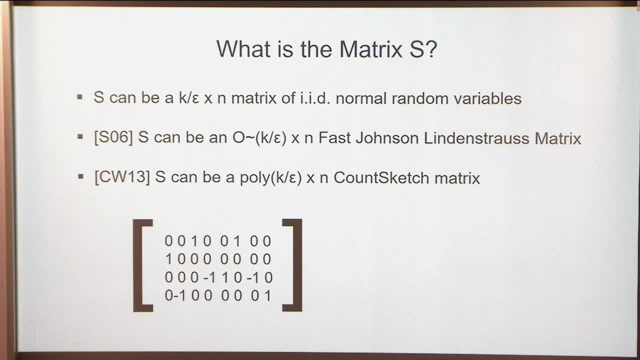 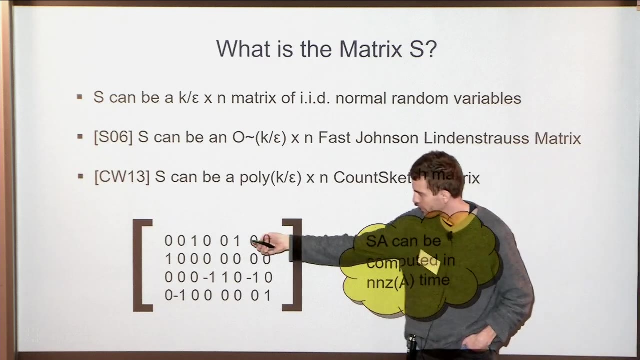 independently for each of the n columns. And the nice thing about this count sketch matrix S is that S times A can be computed in n and z of A time. So for each column of A, for each non-zero entry of that column, it corresponds to a column of S And there's only a single. 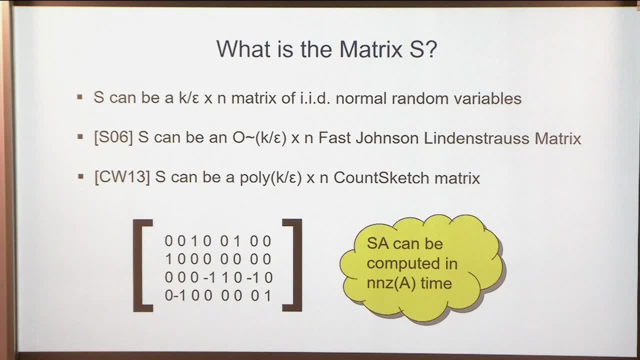 non-zero entry in that column. So I can update the matrix product S times A And you can show that this approach of using sketching for low-rank approximation turns out to give you a good relative error approximation with large probability if the number of rows 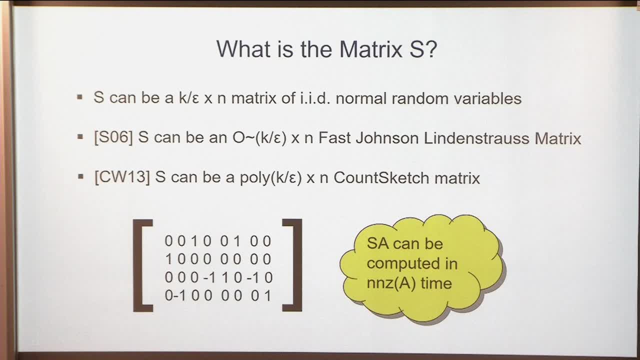 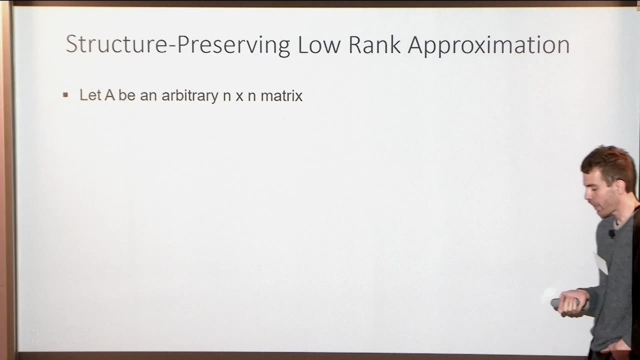 of S is an appropriate polynomial in k over epsilon. So this was the state of the art for using sketching for low-rank approximation. It gives n and z of A time. Recently, what we've been looking at is what I call structure-preserving low-rank approximation. 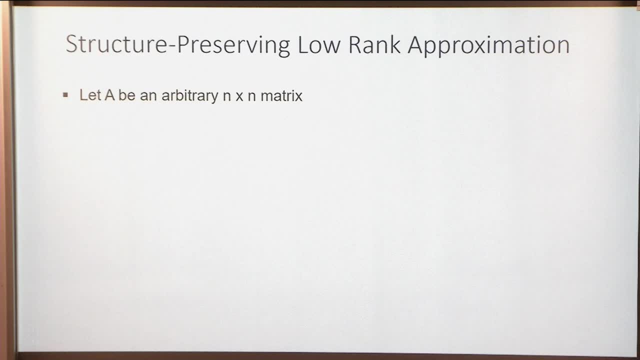 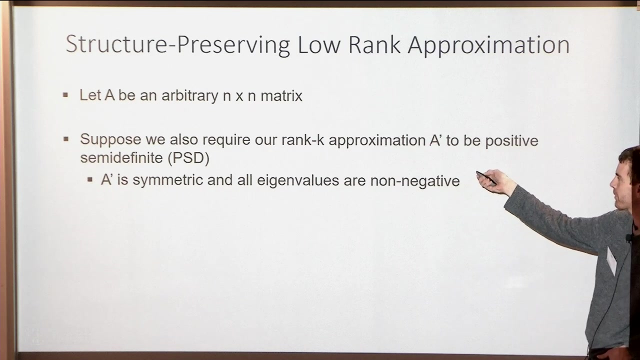 So now let A be an arbitrary n by n matrix. Not only do we want a low-rank approximation, a generic low-rank approximation to A, but we also want our low-rank approximation to have a certain structure. OK, So suppose we require our rank k approximation A prime. 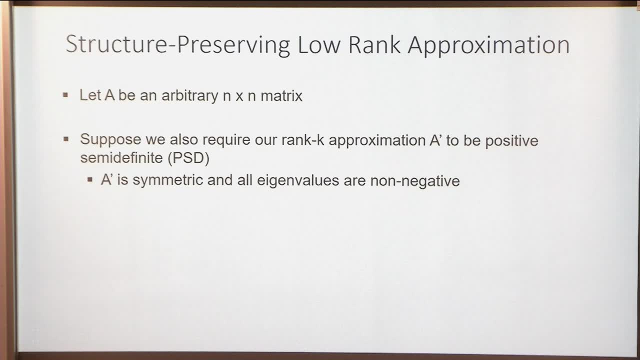 for example, to be positive semi-zero. That's my definite for PSD. OK, So just the definition is that A prime is a symmetric matrix and all the eigenvalues are non-negative. OK, so now can we still solve this problem very quickly. if we require this additional property about A prime, PSD matrices occur. 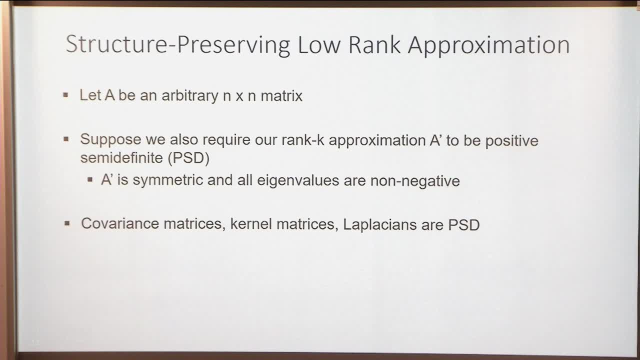 all over the place, For example, covariance matrices, kernel matrices, Laplacians And your matrix A that you want to approximate itself. it needs an auxiliary matrix A, So might not be a PSD matrix, For instance. maybe it was supposed to be a PSD matrix. 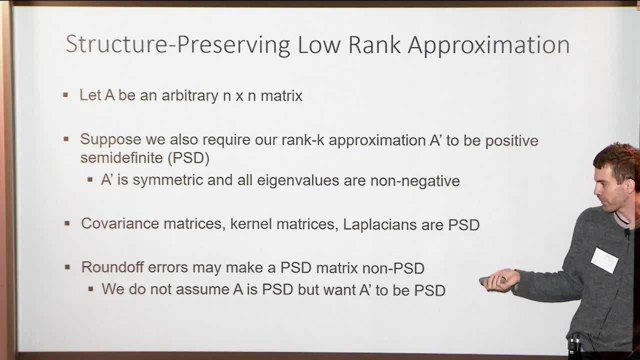 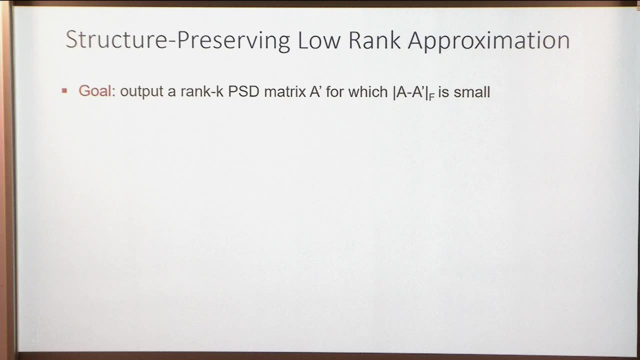 but, because of round off errors in an application, turned out to not be PSD, But still knowing that it should be PSD. you want your low rank approximation, A prime itself, to be PSD. okay, So yeah, so the goal here is just to output. 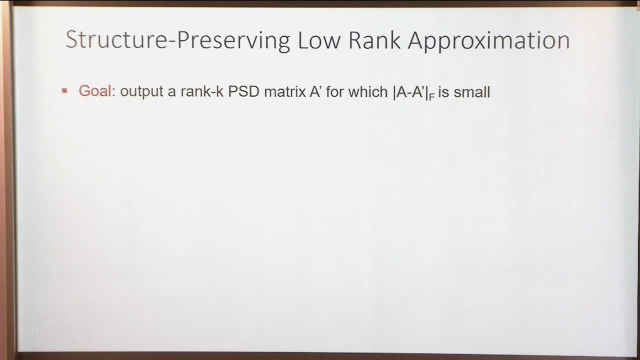 a rank K, PSD. matrix A prime, for which the Frobenius norm of A minus A prime is small. To solve this problem, you can first assume that the matrix A is actually a symmetric matrix. Okay, so right now we have this arbitrary N by N matrix. 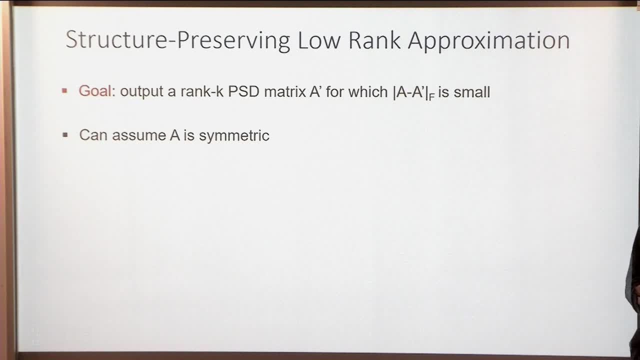 We're assuming nothing about it. We just want a rank K matrix approximating it. And I'm saying that this arbitrary N by N input matrix. we might as well assume it's a symmetric matrix. Why is that? Well, you can write any matrix A. 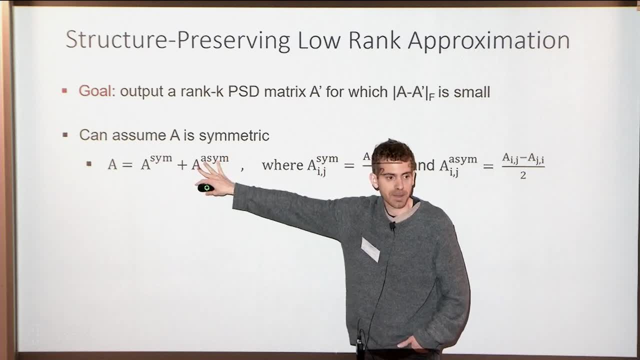 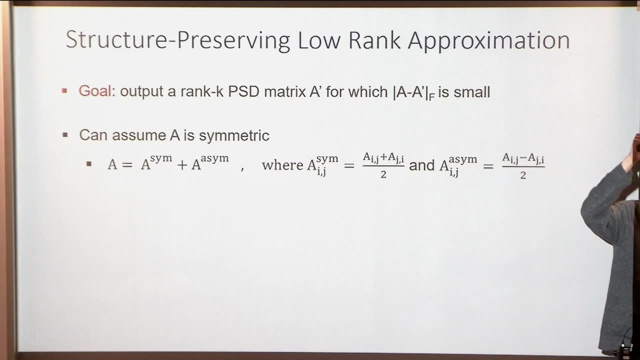 as a symmetric part- A sym, plus an anti-symmetric part, A A sym. How do you do this? Well, the symmetric part is just obtained by averaging the corresponding pair of off-diagonal entries, Aij plus Aji over two. 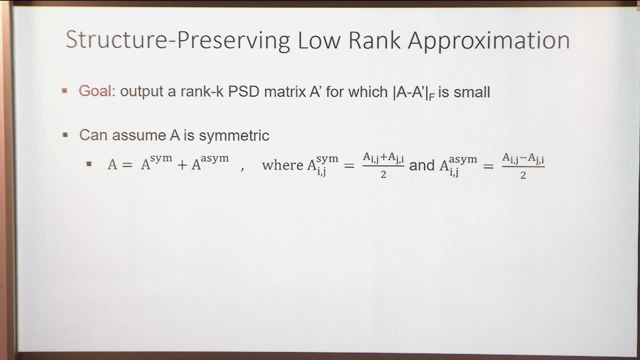 And the asymmetric part is obtained by taking the difference of the off-diagonal entries divided by two. And the important point is that an asymmetric matrix- if you think of it as a vector, it's orthogonal to a symmetric matrix If you think of that as a vector. 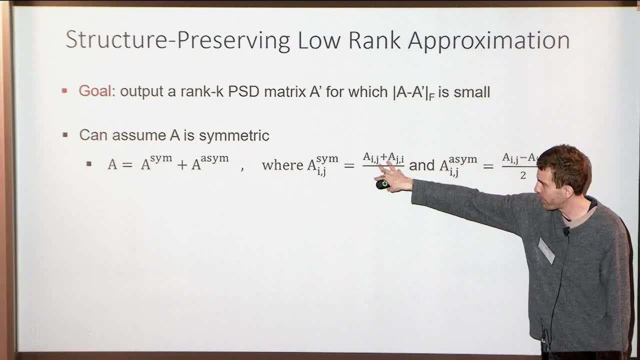 because you'll have two corresponding entries that are equal in the symmetric matrix, but in the asymmetric matrix they'll have opposite sign, So the inner product will be zero And because of that, if I'm approximating A by a symmetric matrix, A prime. 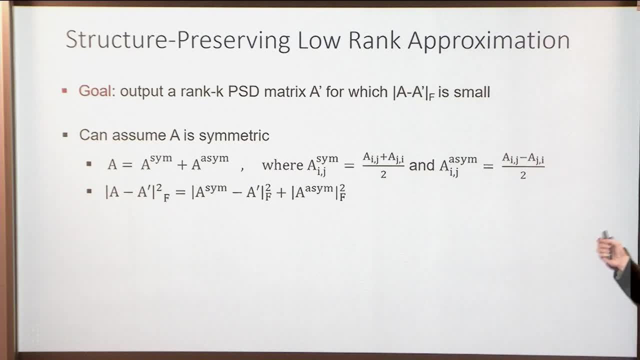 then by the Pythagorean theorem I can write the squared Frobenius norm of A minus A prime as the symmetric part of this matrix, which is A sym minus A prime, The squared norm of that plus the squared norm of the anti-symmetric part of the matrix. 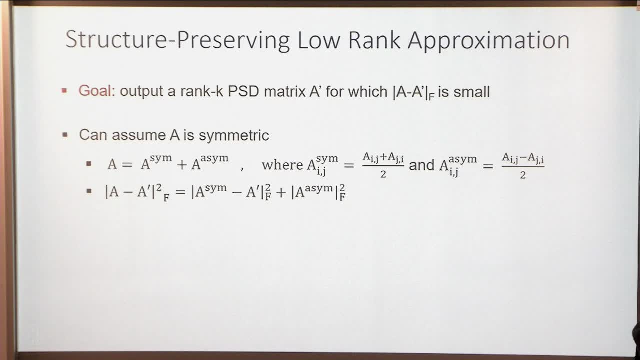 Okay, this is just the Pythagorean theorem, since these are orthogonal, And notice that this second part doesn't even depend on A prime. you know the rank K matrix that you're trying to find, So any rank K matrix, A prime that you find. 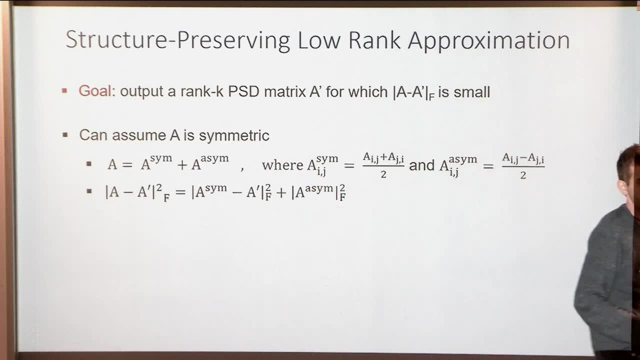 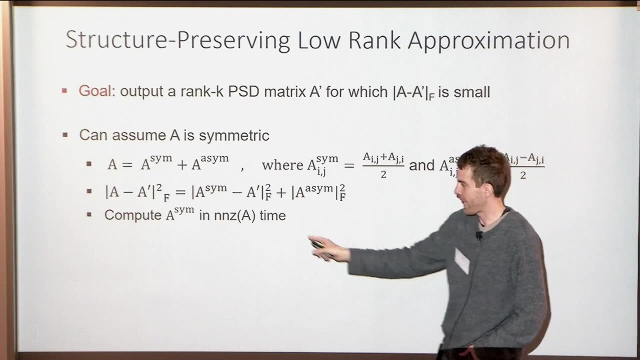 is going to have to pay the cost of this second part, So I might as well just assume that my input matrix A is symmetric, because I can compute it the symmetric part in n and z of A time right. I just average the off-diagonal entries. 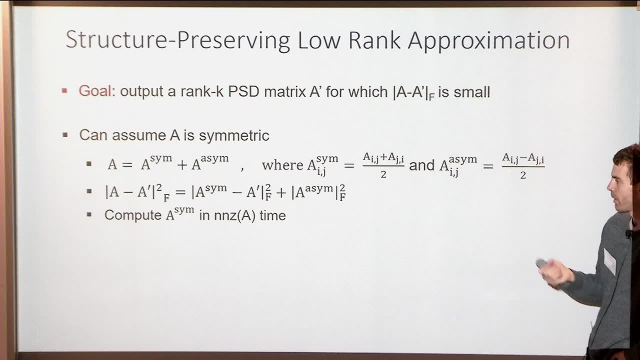 and now I have a symmetric matrix. Okay, so A is symmetric. And what is the best? PSD rank K approximation, which I'm going to call A sub K plus to this matrix A. So if I give you an arbitrary symmetric matrix A, 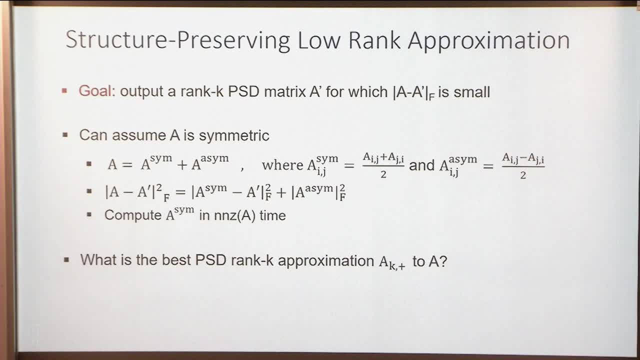 can you tell me what it's? the best rank K PSD approximation is? So you stop at the first eigenvalue, that is, If the last is non-negative or the Kth one, whichever one comes sooner. Yeah, I mean. so you zero out. 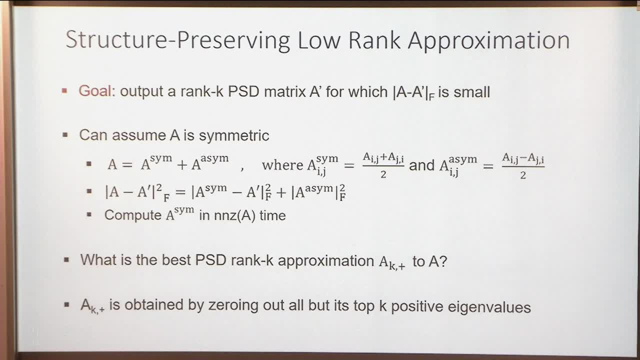 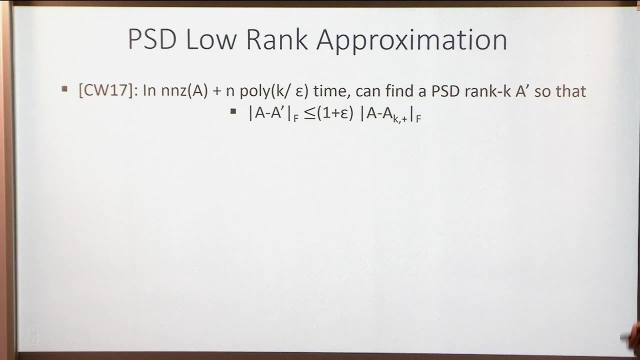 all but the top K positive eigenvalues of A, And that gives me, yeah, A sub K plus Okay. so what is known about this? This is a problem. So in earlier work this year with Clarkson we showed that you can still get input sparsity time. 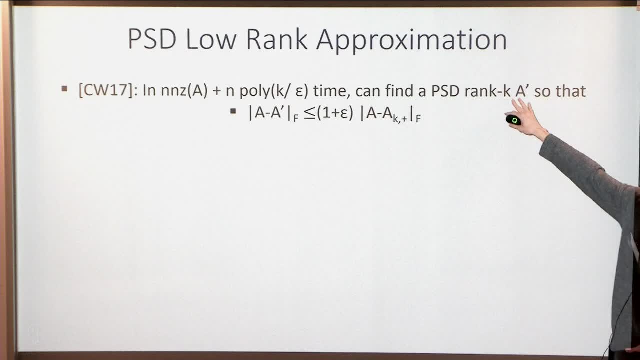 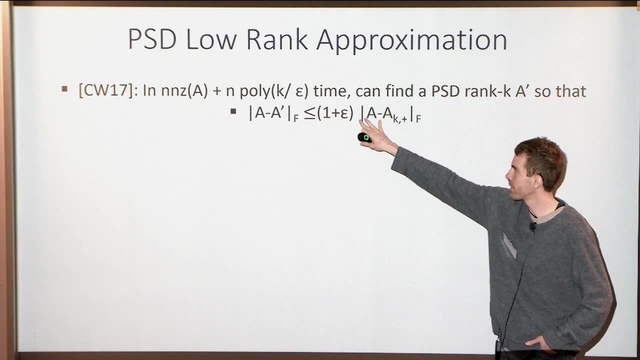 And you can find PSD rank K matrix, A prime which has this relative error guarantee. So the cost is at most one plus epsilon times the cost of using this optimal A sub, K plus. And this improves several previous works. So one thing you might be familiar with. 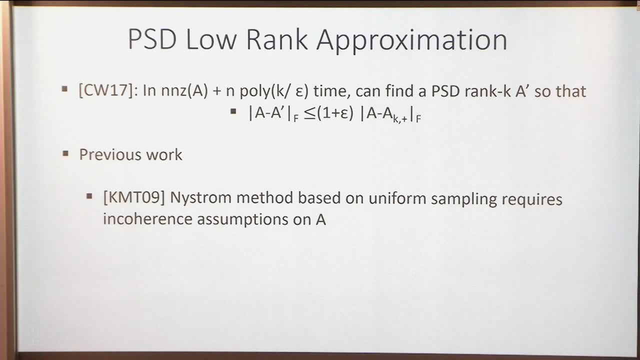 is what's called the Nystrom method, which is a method which occurs in kernels and machine learning. So this is a very fast method, but it doesn't have provable guarantees. It's based on sampling columns of A And, in order to get provable guarantees, 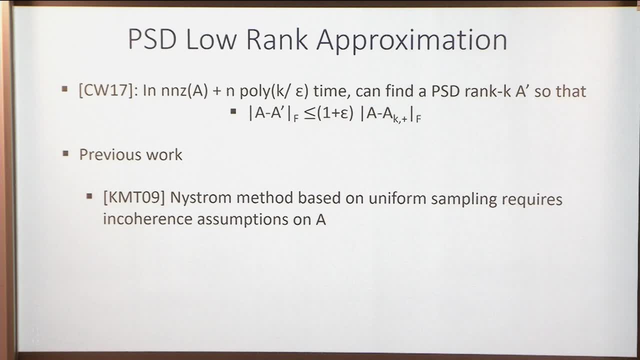 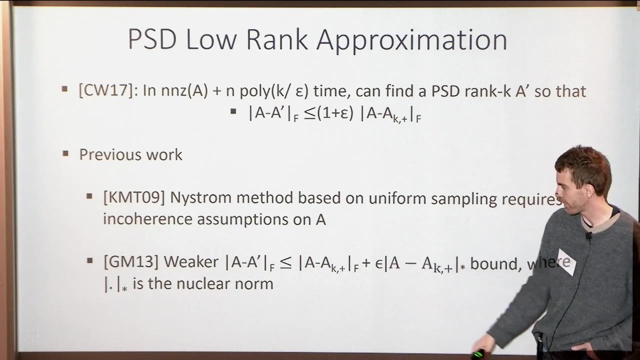 you need to make incoherence assumptions on your input matrix A, Whereas our running time statement holds for an arbitrary A. There's also a bound by Giddens and Mahoney which show that you can find a PSD A prime with a weaker error guarantee. 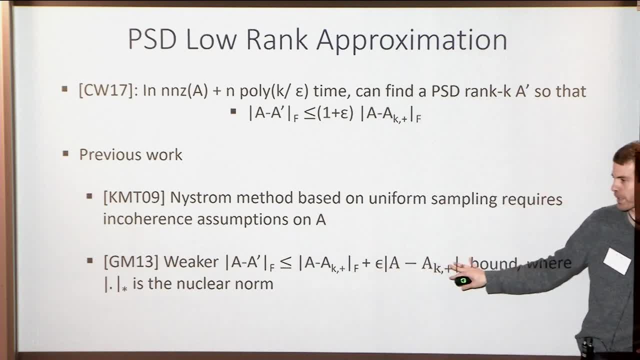 So the error, instead of being epsilon times the Frobenius norm of A minus the optimal matrix, is epsilon times the nuclear norm, the sum of the singular values instead of the sum of the squares, which can be quite a bit larger. 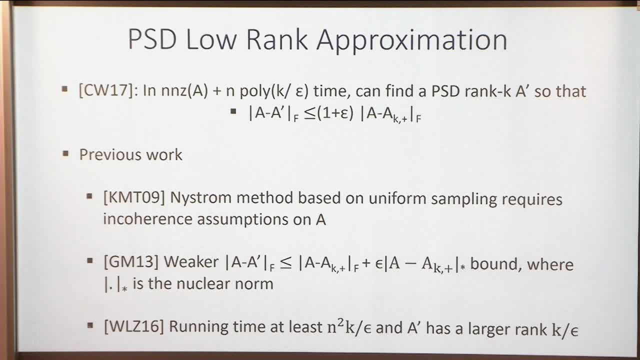 There's work by Wong et al that gets a bit worse of a running time, roughly N squared K over epsilon time and has a larger rank, K over epsilon. Okay, so this is input sparsity time for PSD: low-rank approximation. 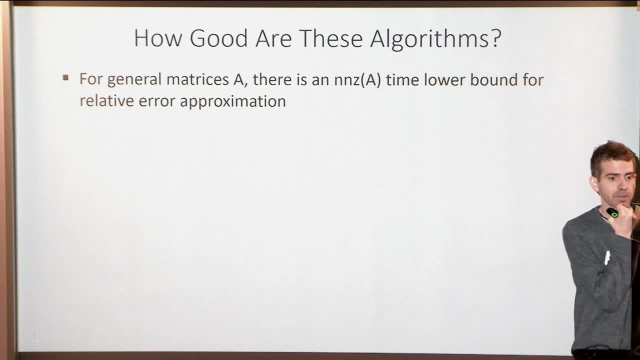 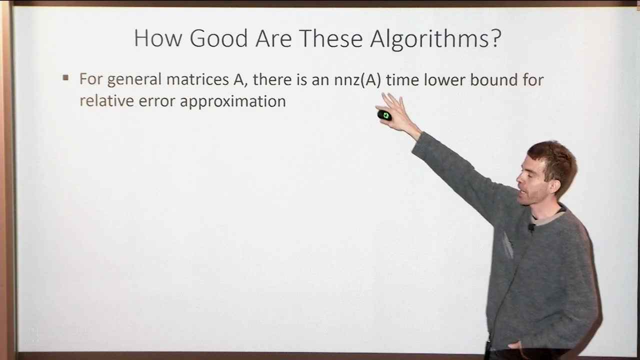 And so the question is: how good are these algorithms? So for general matrices A, there is an N and Z of A time lower bound. You have to read almost all of the entries if you wanna get a relative error. low-rank approximation. 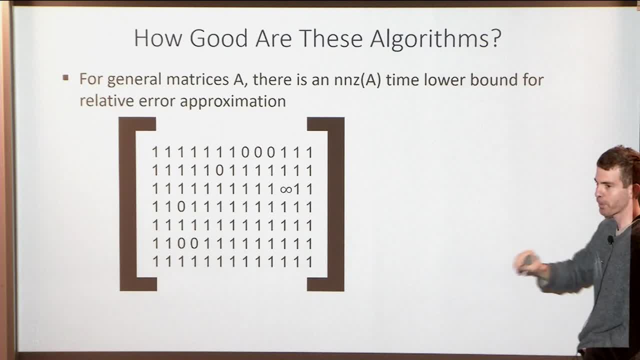 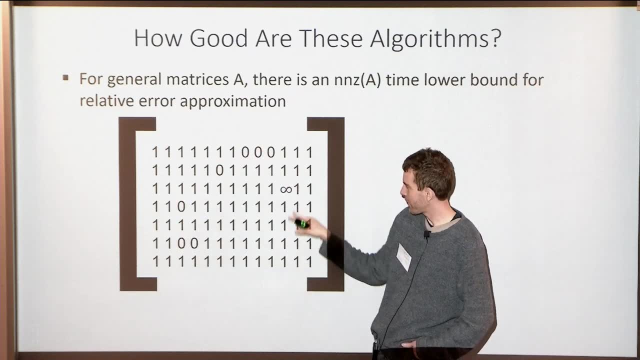 Now, why is that? Well, this is a very simple example. matrix A. It has a bunch of ones and it has some zeros, and one of these entries is infinity Okay, and it's placed at, say, a uniformly random position. 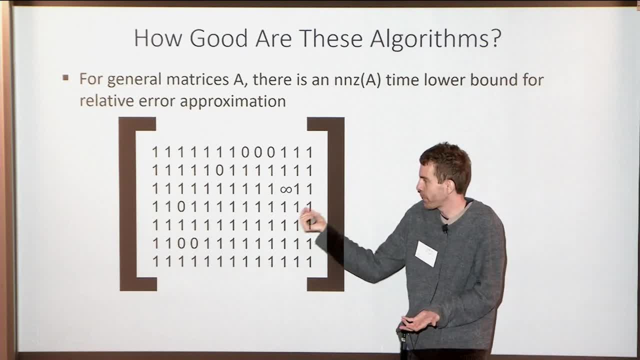 And you have no idea where this entry is. if you don't read most of the non-zero entries, then you're not going to find this infinity entry with large probability. But if I'm a good rank one matrix, you know, the first thing I'm gonna do is I'm gonna assign 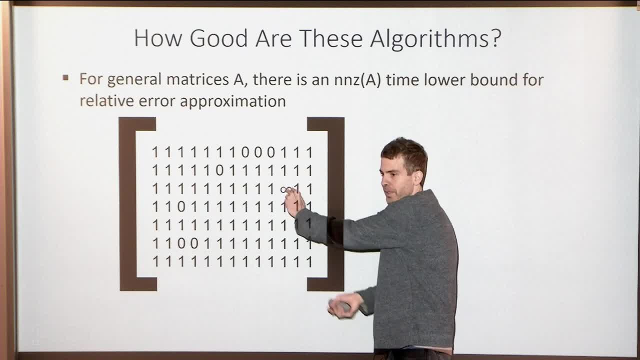 you know, the first thing I'm gonna do is I'm gonna assign. you know, the first thing I'm gonna do is I'm gonna assign infinity to this entry. you know, because I'm taking the difference of this in a rank one matrix. 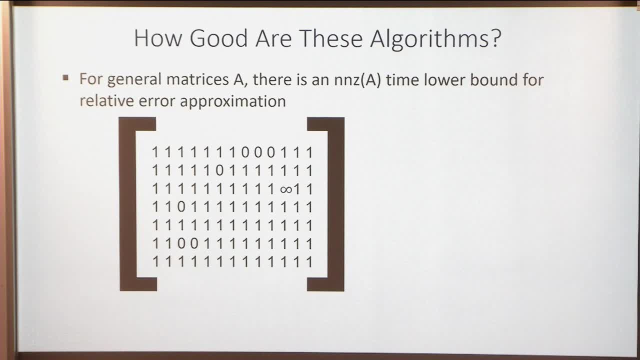 I better wipe out that infinity term. So I need N and Z of A time if I want a good relative error approximation And you can actually show that there's also an N and Z of A time lower bound, even if you require outputting a PSD matrix. 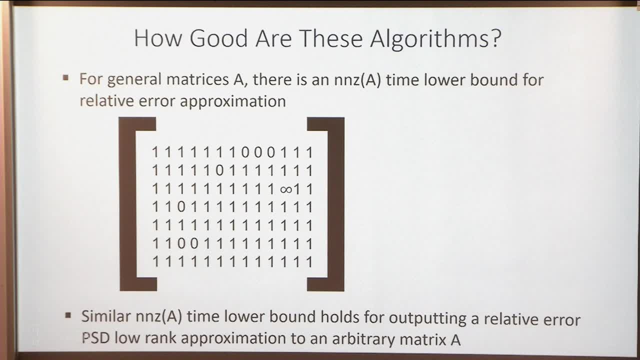 to an arbitrary input. matrix A: Okay. so in fact, these lower bounds, they're even for an easier problem of just someone gives you a matrix A and asks you what is the norm of this matrix? I mean, I still have to read N and Z of A entries. 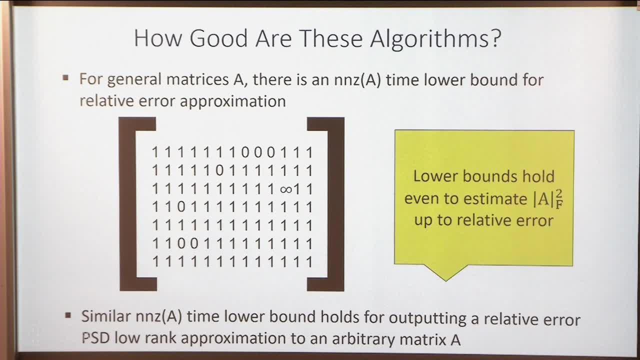 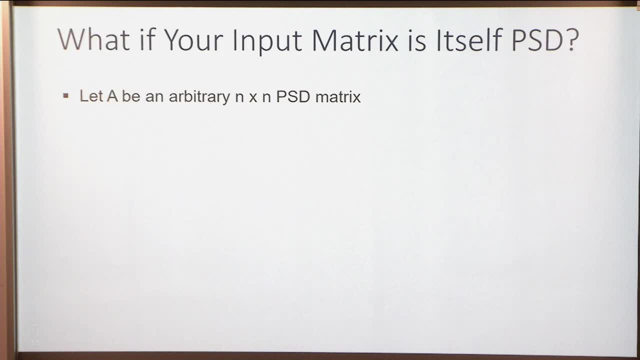 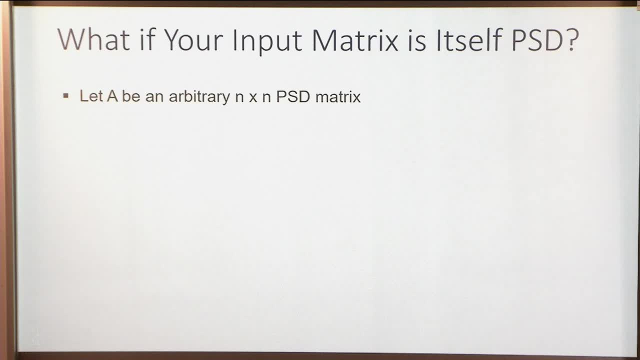 Right. so earlier we were trying to approximate an arbitrary matrix by a PSD matrix. Now our input itself is PSD And maybe we just want to approximate a PSD matrix for efficiency reasons. The question is: is there an N and Z of A time lower bound? 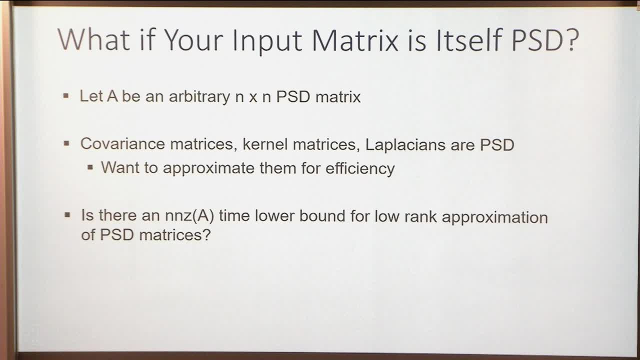 for low rank approximation of PSD matrices? Or stepping back to this even easier question: Is there an n in z of a time lower bound? just for estimating the norm of a PSD matrix, You might only need the diagonal. You might need the diagonal to get an idea of the lower bound. 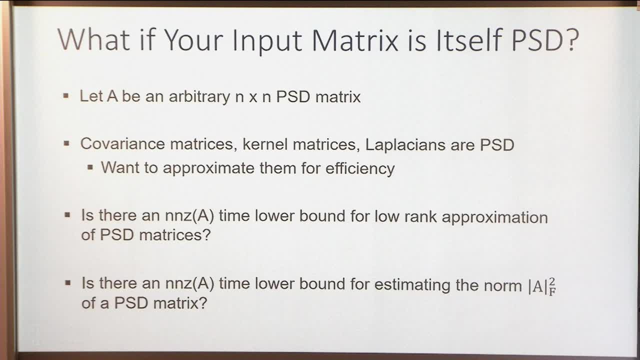 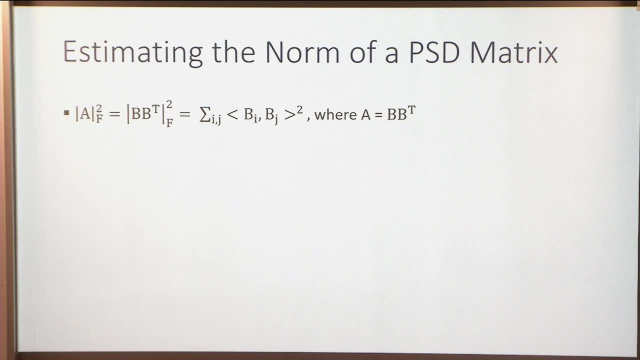 Yeah, so the diagonal is very key to this problem and that's the right intuition. And it turns out that you can estimate the norm of a PSD matrix reading roughly only order n entries. Okay, so let me just give you know this will help for intuition, for the low-rank approximation. 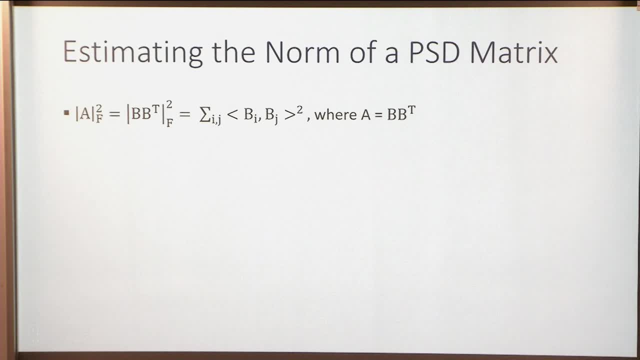 So let's see how to estimate the norm of a PSD matrix in sublinear time. So I'm looking at the squared Frobenius norm of some PSD matrix: A, Now A is PSD, which means that I can write it as B times B transpose. 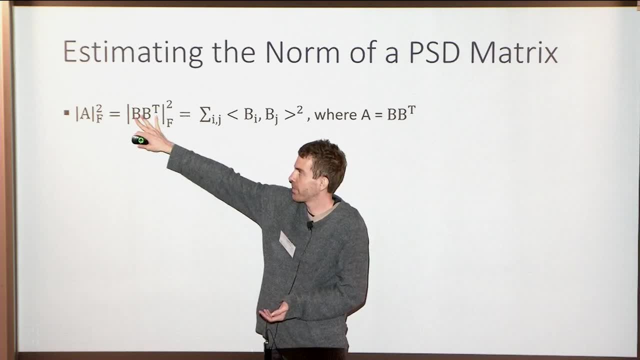 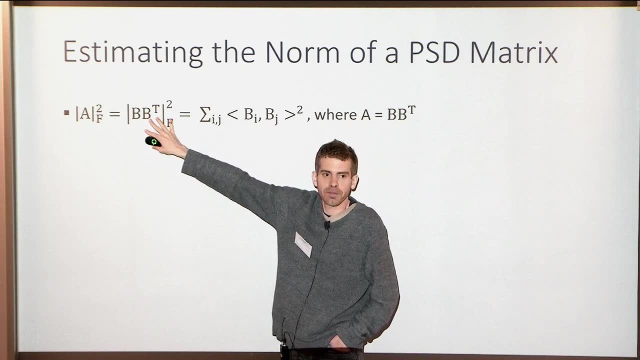 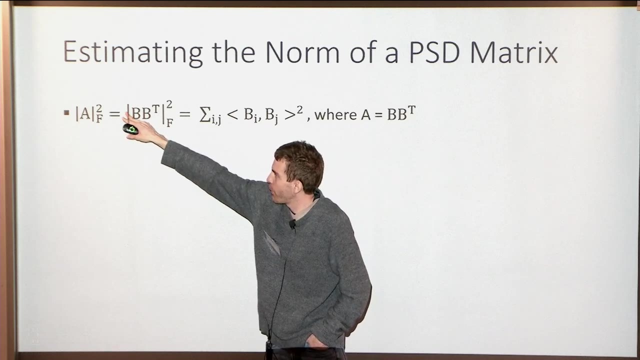 But I can think of B as being the square root of A. This is well defined, since A is PSD. So what is the squared Frobenius norm of B? B transpose, That's the sum of squares of all the entries. Well, what is the ijth entry? That's just the inner product of the i-th row of B and 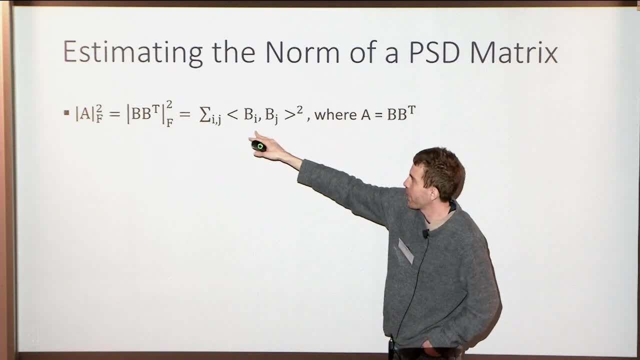 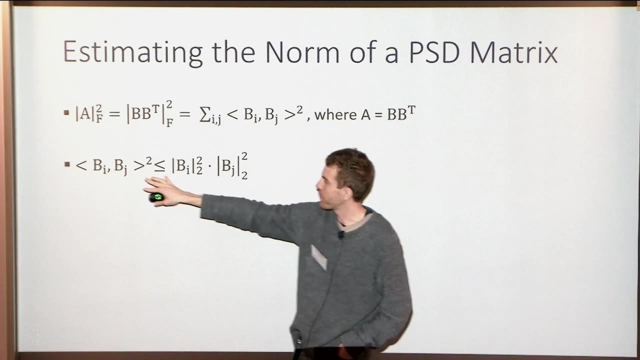 the j-th row of B, right The j-th column of B, transpose- And I'm looking at the sum of squared entries: Okay, Well, what do we have So by Cauchy-Schwarz, let's look at one of these entries. 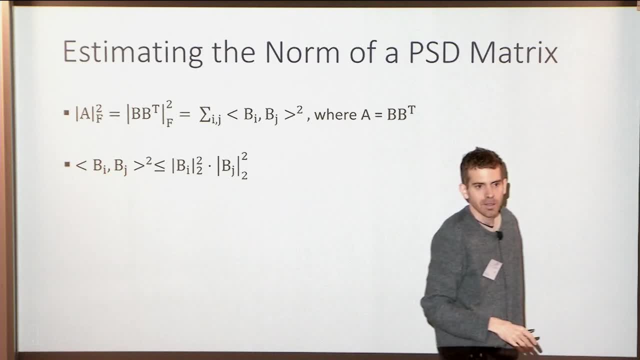 the inner product of B i, B, j squared By Cauchy-Schwarz. this is at most the squared norm of B i, the i-th row of B, times the squared norm of the j-th row of B Right. And what are these entries? 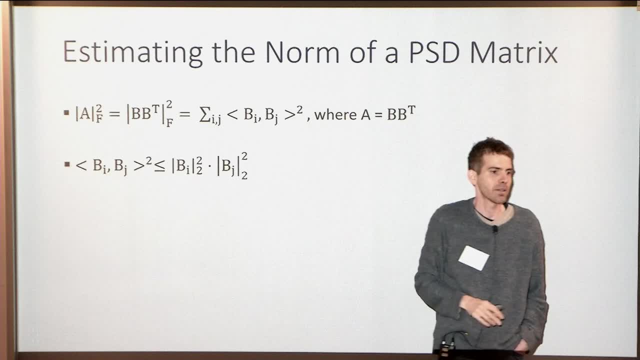 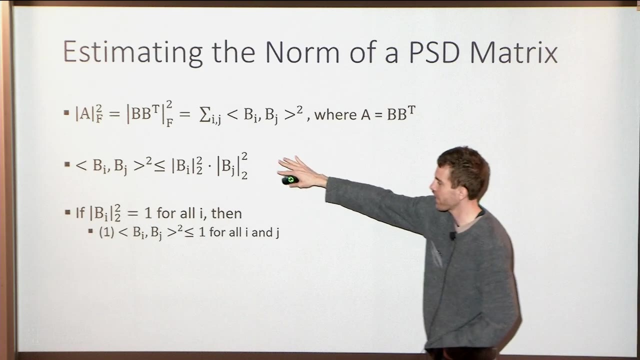 These are the diagonal entries of A Right. So Okay, so suppose all the diagonal entries of A were 1, just for some intuition. And what does this statement mean? Well, this Cauchy-Schwarz is then saying: well then, all the off-diagonal entries have to have absolute value, at most 1.. 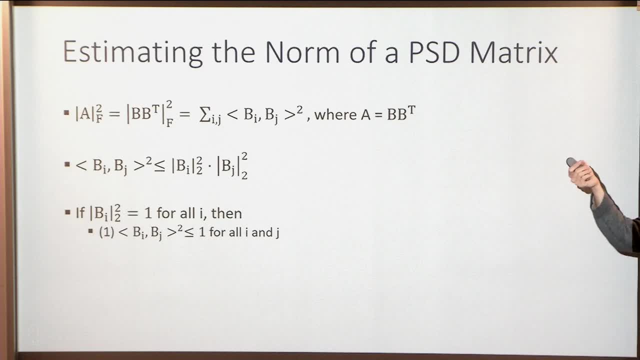 So now I can't hide this infinity in an off-diagonal entry, because it means that one of the diagonal entries must also be infinity. And now let's suppose the sum of squares of the off-diagonal entries actually contributed a lot to the Frobenius norm. 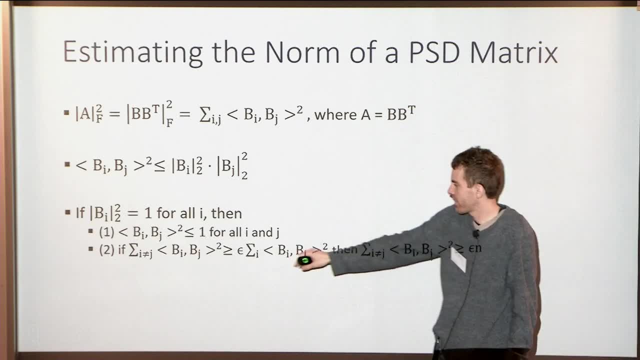 Of A, In particular it was lea-, the sum of squares of the off-diagonal entries was at least an epsilon fraction of the overall Frobenius norm, which means: suppose it's at least an epsilon fraction of the contribution to the Frobenius norm on the diagonal alone. 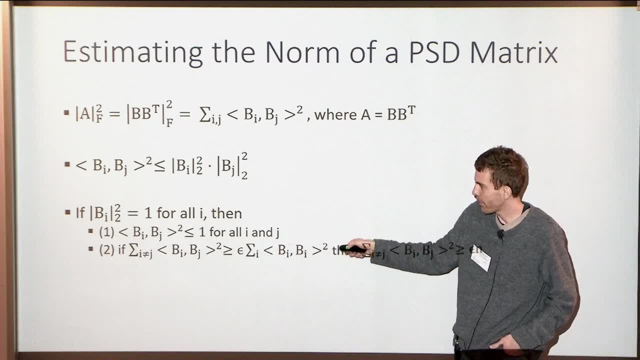 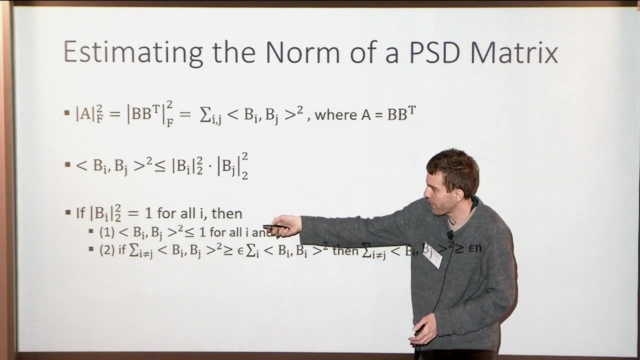 Well, all the diagonal elements are 1.. Right, That was just by assumption. This is 1.. So this means the sum of squares of off-diagonal elements is at least epsilon times n. If it's not, then it doesn't matter. Like if we know, the sum of squares of the diagonal elements is n. every diagonal element is 1.. 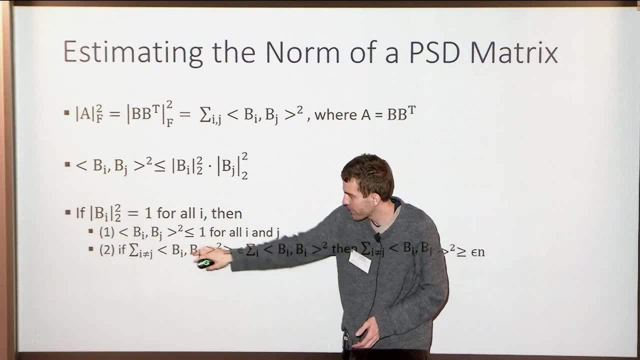 And if the off-diagonal elements, if their sum of squares contributes to the overall squared Frobenius norm, well, its sum of squares had better be at least epsilon n. If it's smaller, then we don't even need to look at the off-diagonal elements. 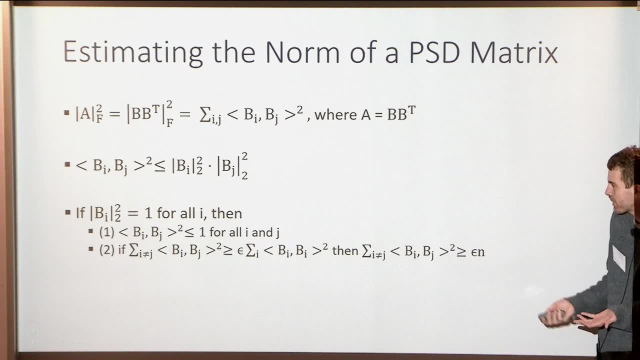 Okay, but now we're in a situation where we have a bunch of small terms. All of these terms- i, b, j, inner products squared- are at most 1. And they sum up to something very large like epsilon n. 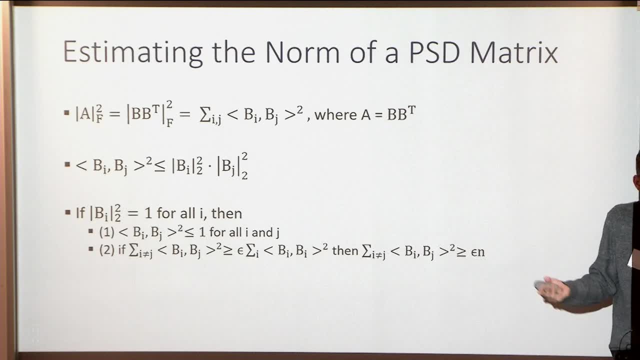 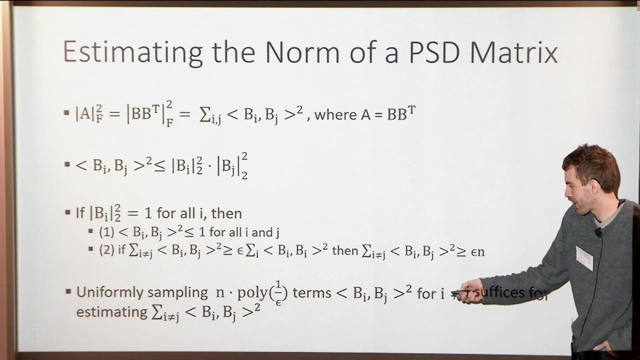 So what do you do when you have a bunch of small things summing up to something very large? Yeah, so uniformly sample, right? So uniformly sampling, if we sample roughly n times a polynomial and 1 over epsilon of these off-diagonal terms. 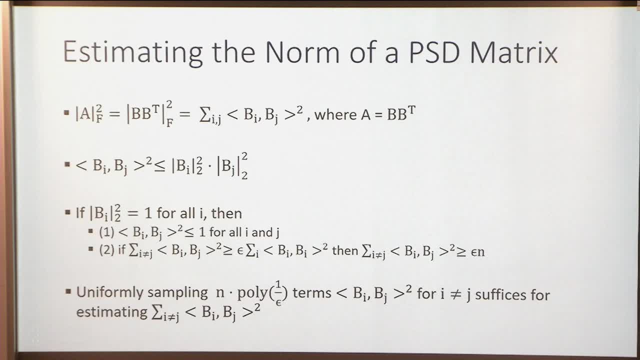 you know, we average them and then we scale back up by the reciprocal of the sampling probability. we get a good feeling, we get a good estimate for the sum of squares of the off-diagonal terms. So we only had to sample n off-diagonal terms. 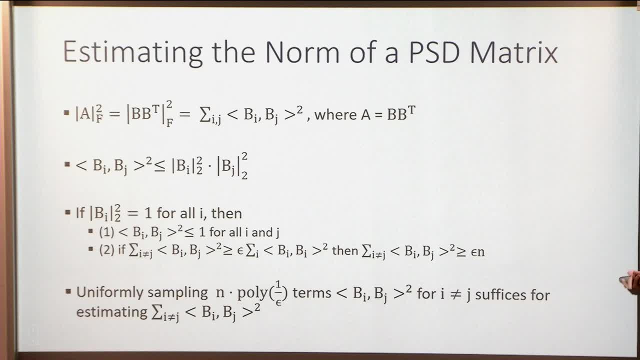 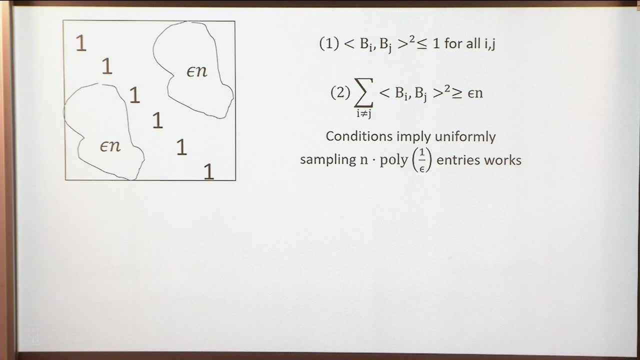 and that's it. So we had an order n sublinear time algorithm. So just pictorially, we were assuming that the diagonal entries were all 1, the sum of squares of off-diagonal entries was at least epsilon n, and each off-diagonal entry is at most 1 in epsilon. 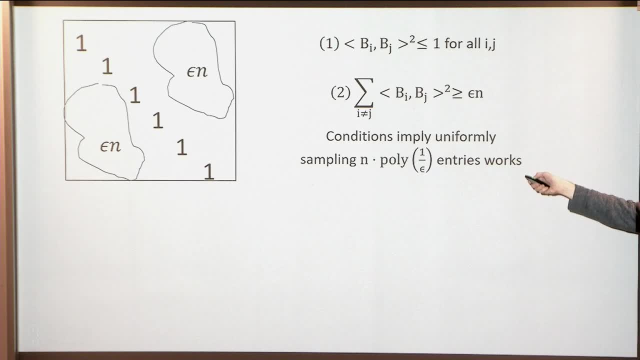 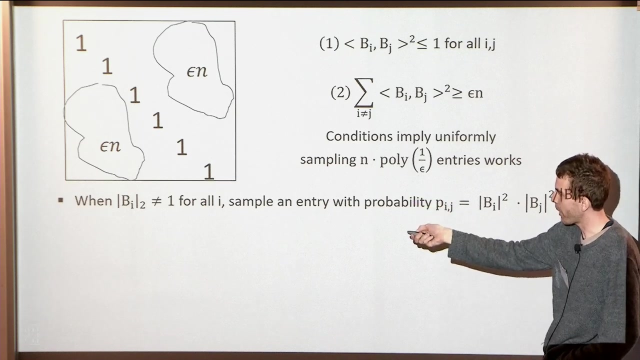 That's an absolute value. These were these two conditions And they imply that uniformly sampling entries gave me a good approximation to the squared Frobenius norm. And something very similar happens when the diagonal entries are not all equal to 1. You just do importance sampling instead of uniform sampling. 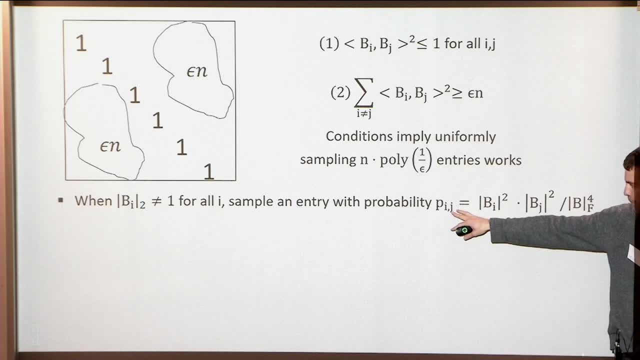 So just quickly define the probability pij of sampling an entry, ij to be, you know, 1 over epsilon n, And that's it. So pij to be the squared row norm of bi times the squared row norm of bj, divided by a normalization factor. 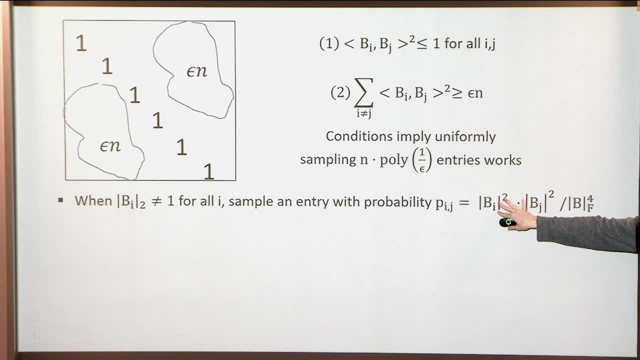 This factor is the sum of squares of all of these. So notice that this probability, pij, can be computed just by reading the diagonal entries right. This is the i-th diagonal entry of A, This is the j-th diagonal entry and this is the sum of all of them. 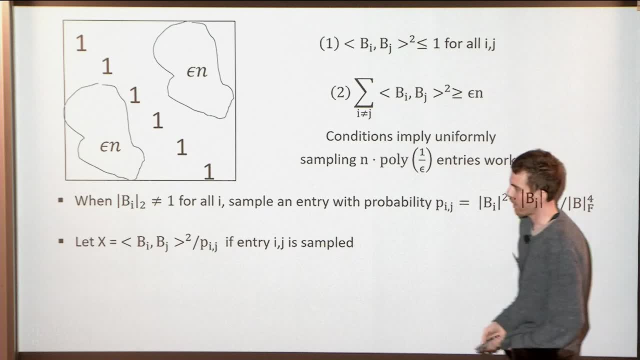 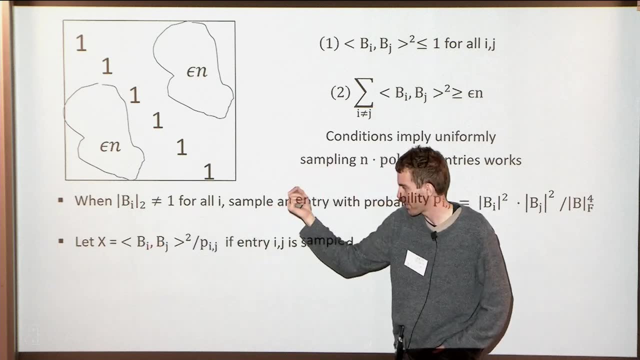 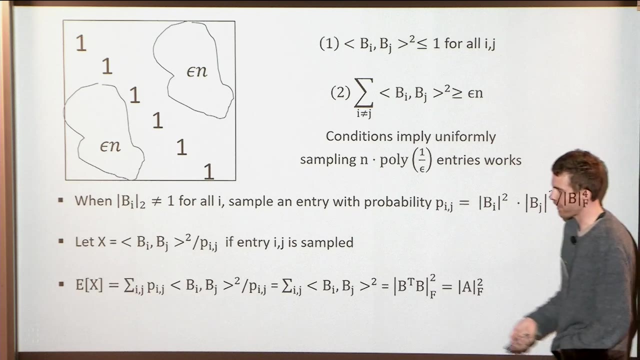 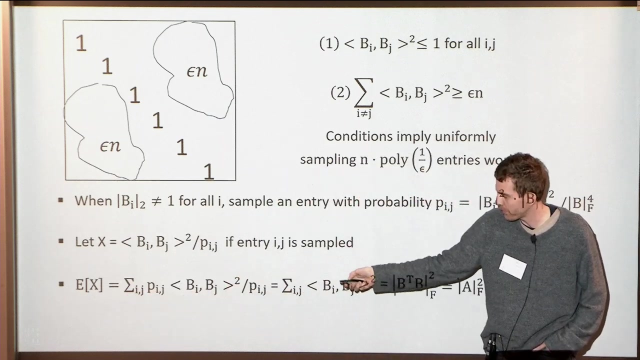 So if I just do importance sampling, if I just let my random variable x be the squared value of the i-j-th entry divided by the probability of sampling it, then just the standard thing here is that the expectation of x is the sum over all entries, ij of the probability of sampling, the entry times, the squared value over the probability of pij. 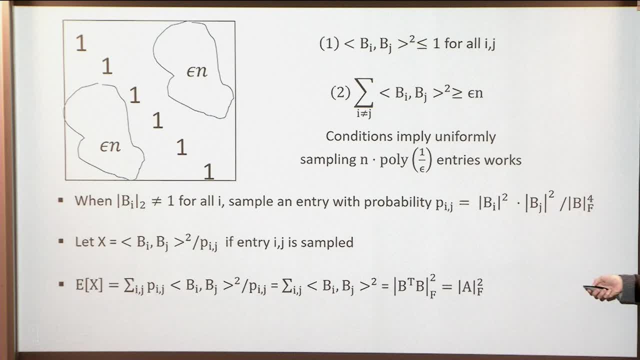 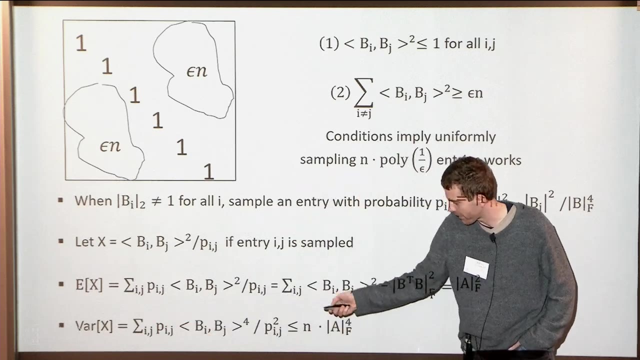 This is my random variable. if I sample it And I get that the expectation is the squared value. This is the squared norm And I can upper bound the variance by this second moment And it's just the sum over all ij of the probability of sampling that entry times the squared value. if I sample that. 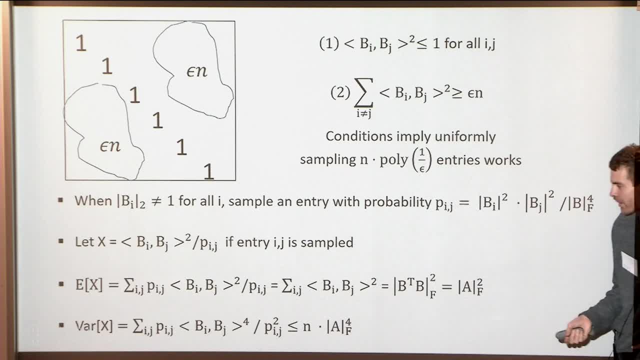 And now I just use the fact, this Cauchy-Schwartz, again. I cancel one of the probabilities and I use Cauchy-Schwartz to upper bound this inner product in terms of the squared norms of the rows, And so I can, overall, you can show that the variance is, at most, n times the squared value. And so I can. overall, you can show that the variance is at most n times the squared value, And so I can. overall, you can show that the variance is at most n times the squared value, And so I can. overall, you can show that the variance is at most n times the squared expectation. 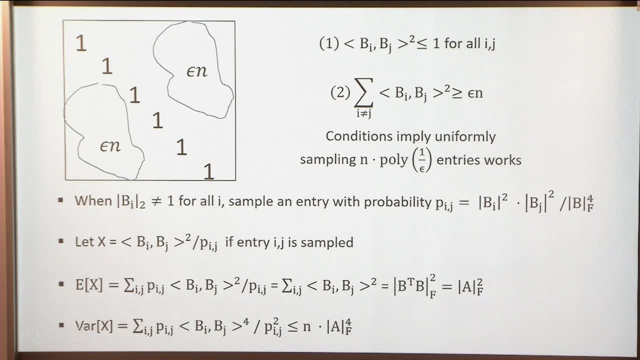 And so I can. overall, you can show that the variance is, at most, n times the squared expectation. So this means that if I take, you know, roughly n samples, I'll get a good approximation with high probability- Okay, I mean with good probability. 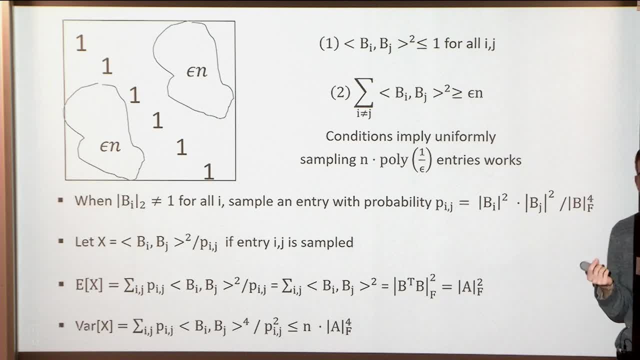 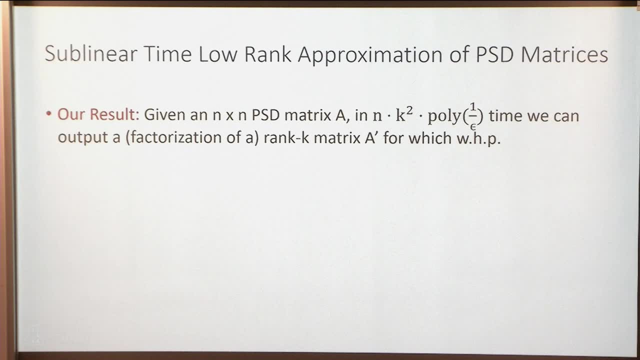 Okay. so PSD matrices: it's possible to estimate their norm And um. So the previous lower bound strategy doesn't apply, And our main result is actually that, given an n by n PSD matrix in raghfully n times k, squared pi. 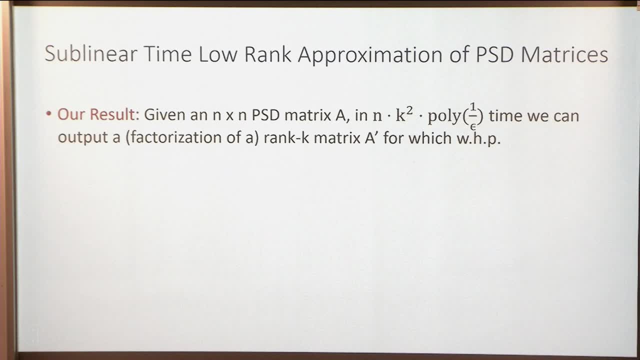 in raghfully n times k squared pi times k squared poly 1 over epsilon time, we can output a rank k matrix, A prime, which achieves relative error that the Frobenius norm of A minus A prime is at most 1 plus epsilon times the optimal rank k approximation cost. 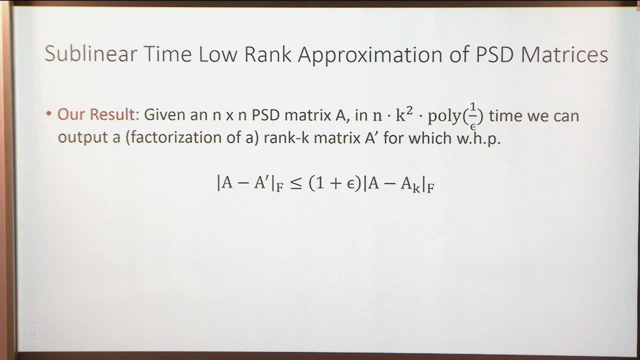 Okay, so this is much faster than these input sparsity time algorithms that we saw based on sketching earlier in the talk. This corresponds to, say, one of the low-order terms in those input sparsity time algorithms. In fact, the number of entries we read is roughly about n times k for constant epsilon. 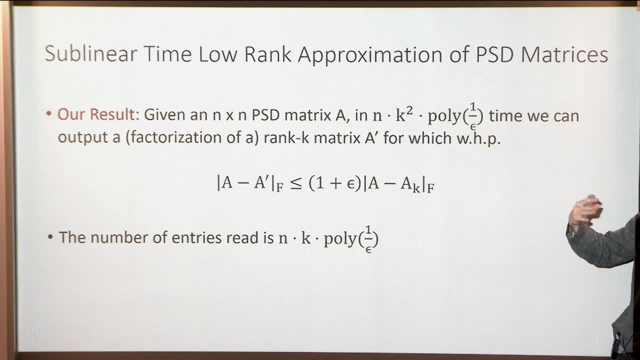 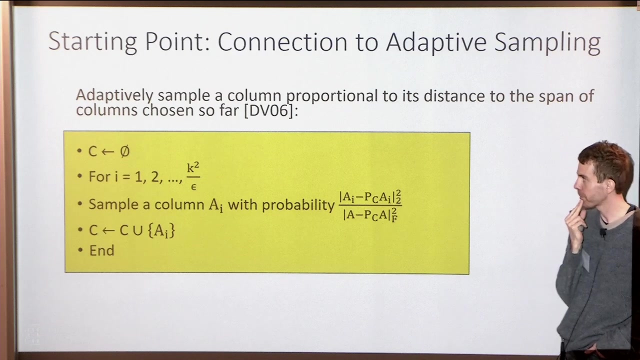 And if the matrix multiplication is 2, we can improve this to n times k, And we do show a lower bound that you need to read roughly nk over epsilon entries. So at least for constant epsilon This is roughly tight. Okay, so let me give you some intuition of how the algorithm works. 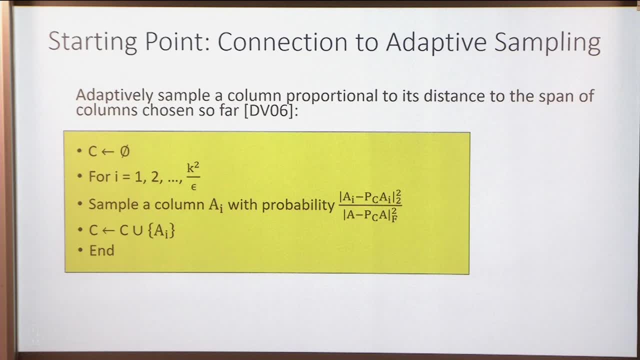 So the starting point is a connection to what's called adaptive sampling, And this is an algorithm proposed by Deschpen and Vimpala. So the idea is as follows: You'd like to You have this n by n matrix A and you'd like to sample a small subset C of its columns. 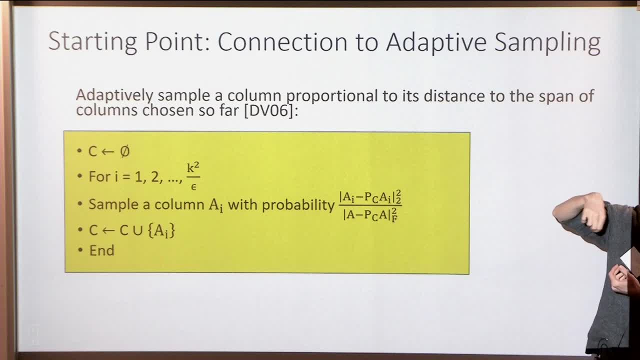 which contains This small subset, contains a good rank k. It contains a good rank k space inside of its span. This is your goal. And how are you going to do this? What you do is you start off. You have no columns chosen and you just choose a column proportional to its squared norm. 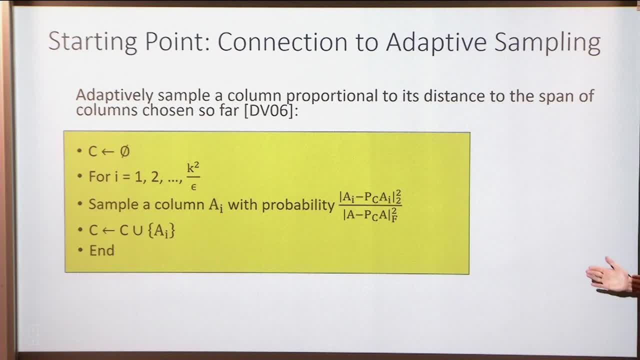 That's the first step. Now I have one column. Now I look at all my remaining columns and I compute their square distance to the column I've already chosen And I sample proportional to that square distance. Now I have two columns. Now I take two columns and I look at the span of these two columns and I look at all. 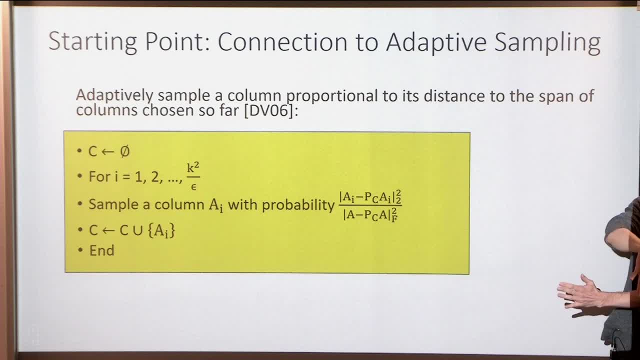 my remaining columns and I sample a column proportional to the square distance of the span of those two columns And I repeat this process. So I iteratively choose a column with probability proportional to its square distance to the span of the columns that I've already chosen. 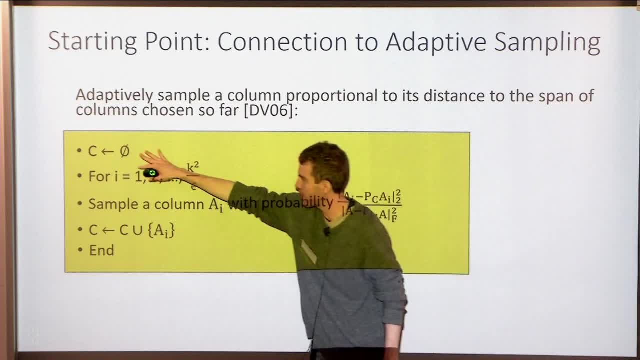 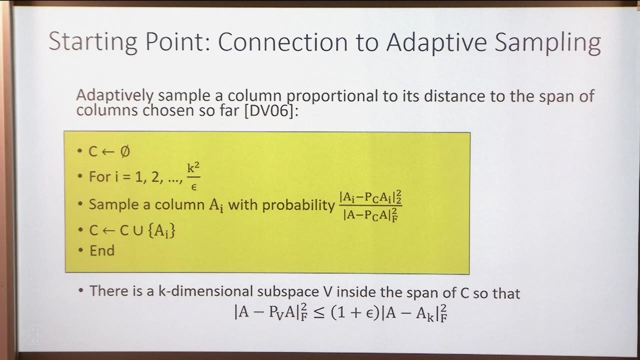 So that's all this is saying. I initialize my columns to empty set and I repeat this process roughly k squared over epsilon times, Just sampling proportional to the square distance, to what I've already chosen. That's what this statement is saying, And what they prove is that if you do this, then there exists a k-dimensional subspace. 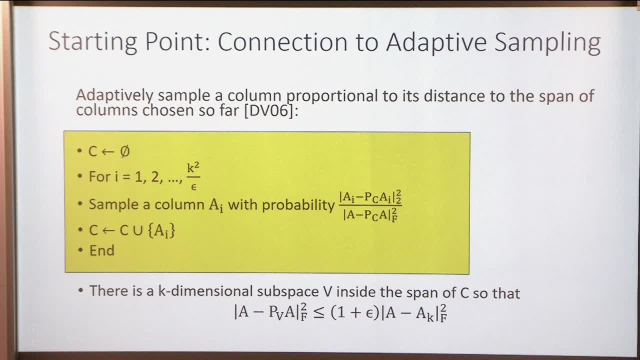 v inside of the span of these roughly k squared over epsilon columns that you sampled, such that if I were to project my columns of A onto this k-dimensional space so I get a rank k matrix, then this is a good rank k matrix. 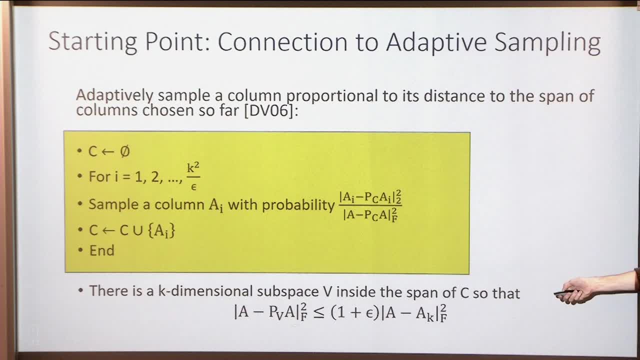 It means that the cost of using that rank k matrix is, at most, 1 plus epsilon times the optimal cost of any rank k approximation. OK, so this was a very simple, intuitive algorithm. but there's something very important to note about this algorithm, which is that it doesn't look at many inner products between pairs. 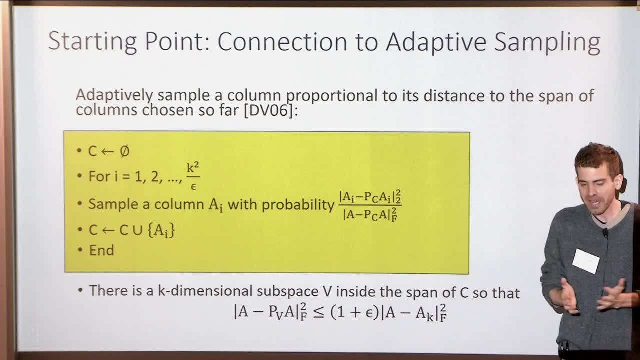 of columns of A. So I have n columns And there are n squared pairs of columns And I could be looking at the inner product between all n squared pairs of these columns. You could imagine algorithms that do that. This algorithm is not doing that. 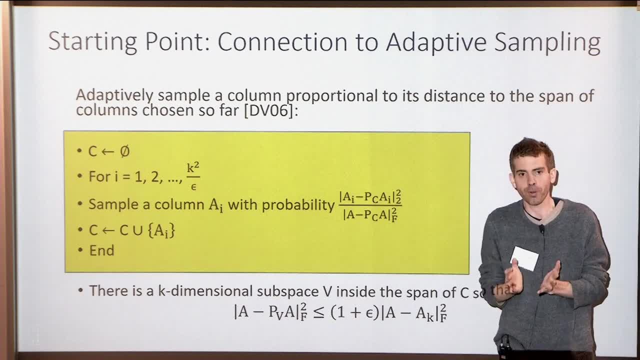 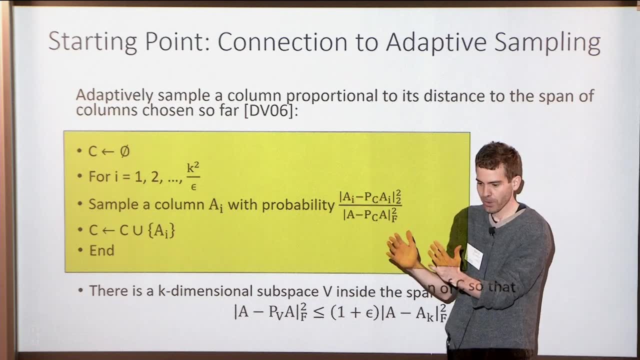 What is it doing? It's actually looking at a very small number of inner products between pairs In the first step. what is it doing? It's just sampling a column based on its squared norm. Well, that's just looking at n pairs of columns, like a column with itself because its squared. 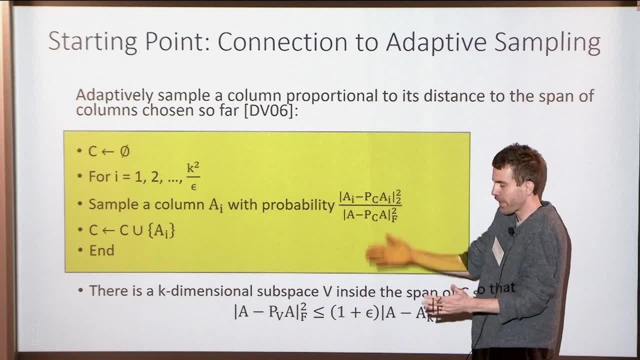 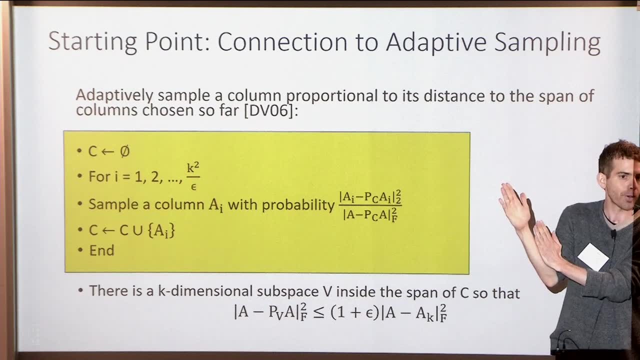 norm is just its inner product with itself. I'm looking at n of these, Then I sample a column. Then I want to look at my remaining n minus 1 columns and find their distance to the column I've already sampled. That just involves knowing the inner product of that column with the column I've already. 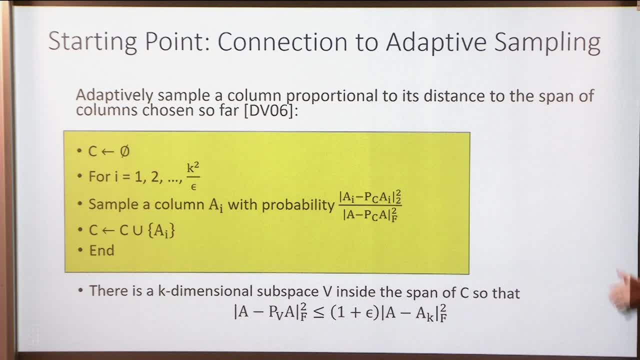 sampled, That's just n more inner products. Now I have two columns And now I need to know these n minus 2 columns. I need to know their inner products. with both of the columns I've already sampled. So, in fact, this algorithm, it only needs. 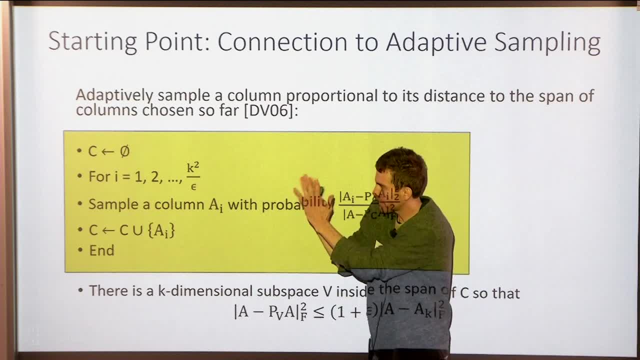 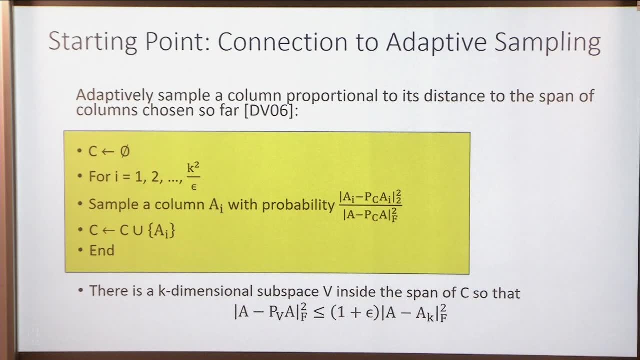 It only needs n times the size of the number of columns, which is k squared over epsilon. pairs of inner products. It only has to look at a very small number of pairs of inner products, of columns of your input matrix. Okay, so this will be a very important property on the next slide. 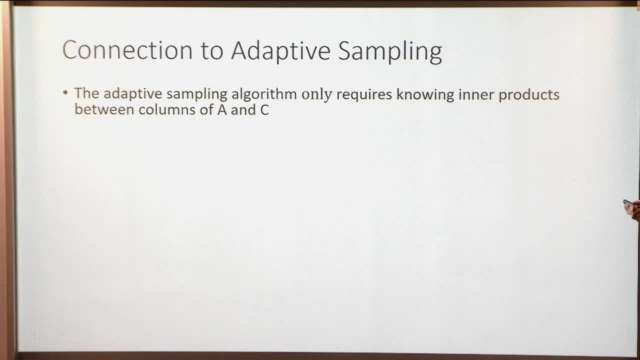 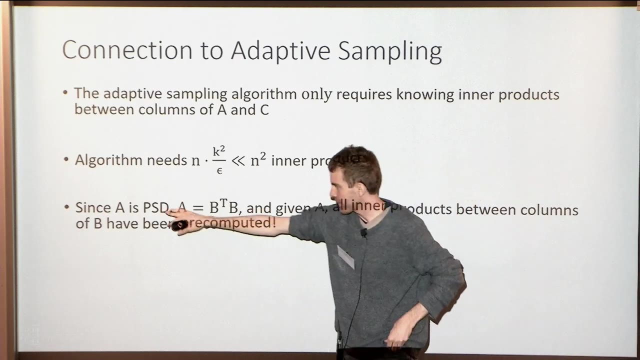 Yeah, so, as I just said, it looks at just The algorithm, only looks at much less than n squared of the total possible number of inner products it could look at. And so the idea I mean. so here's one idea. So again, since A is PSD, we can write it as say B, transpose B, And the nice thing. 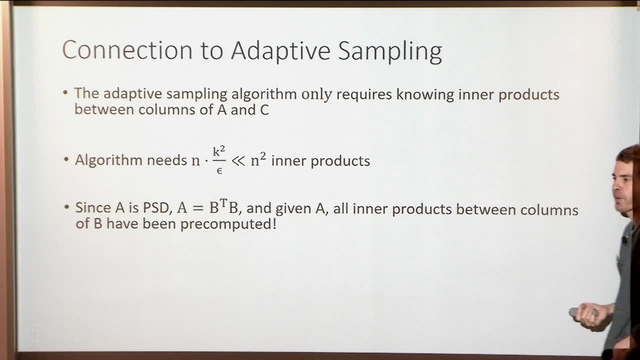 about this is suppose we wanted to run our adaptive sampling algorithm on B. Then A has already come And we're given A, Then A has already computed all the pairs of inner products that we've got. And we're given B, Then A has already computed all the pairs of inner products that we might. 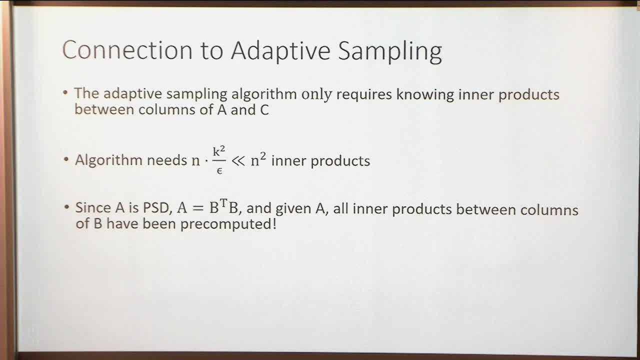 need Right. A is the matrix of inner products of all the columns of B. So what I can do is I can just run the adaptive sampling algorithm on B without actually knowing B. I just read the inner products that I need to run that adaptive sampling algorithm. 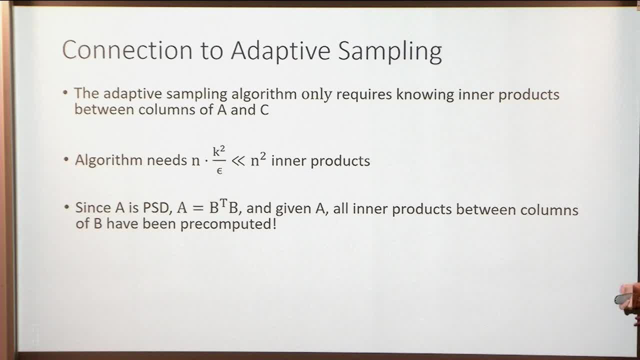 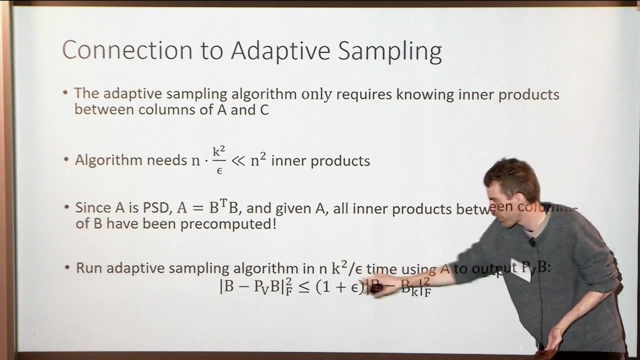 And those inner products are entries of A And we just said: well, we only need to read a very small number of entries to run the whole adaptive sampling algorithm. So I can run this whole adaptive sampling algorithm in sublinear time, roughly n k squared. 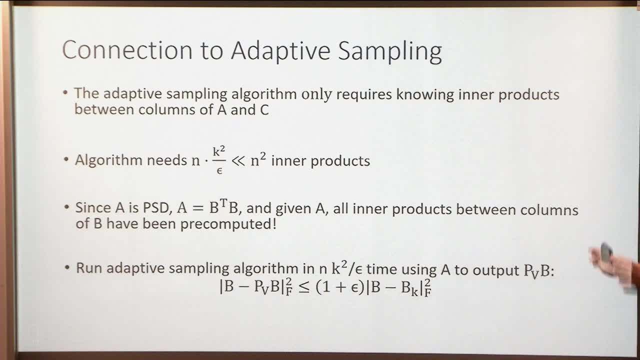 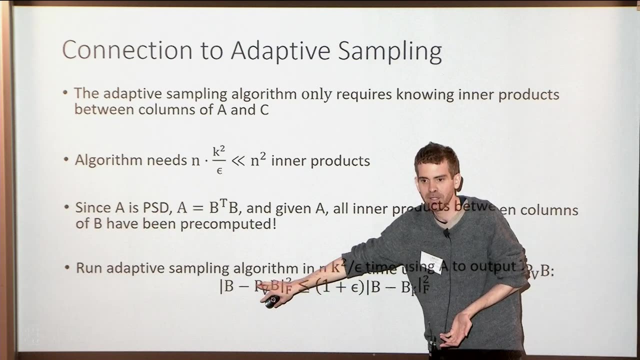 over epsilon time. I just use this matrix A as an oracle whenever I need an inner product for a pair of columns in B. OK, So this will give me an output, a rank k approximation, which is a good low-rank approximation to. 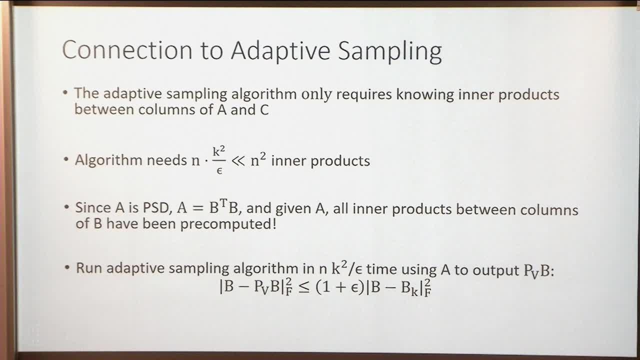 B. I mean, that's the adaptive sampling algorithm that we just said. OK, So A is like this table of all inner products that we might need. The problem with this, though, is we wanted a good low-rank approximation to A, And it. 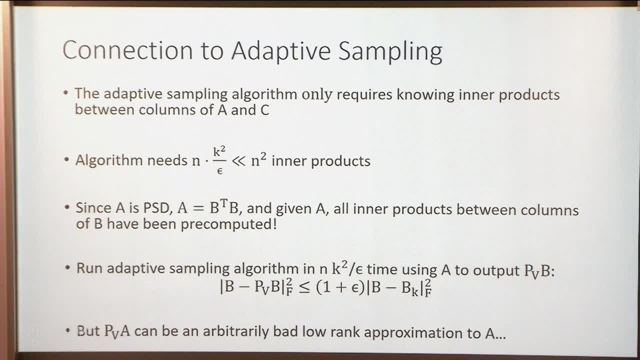 turns out that if you use this same OK, so B and A. B is the square root of A. B and A have the same singular vectors. So if there's no approximation involved, if I took the best rank k space for B, it would: 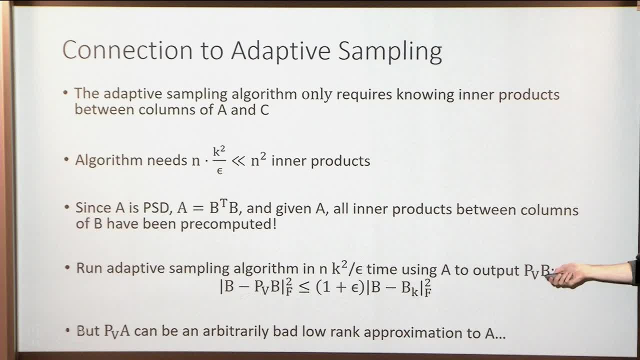 also be the best rank k space for A, But since there's approximation involved- actually this is not approximation preserving. So you can show that this: if you use this same space formed from that small set of columns by running adaptive sampling on B, if you use that same space for A, you can get an. 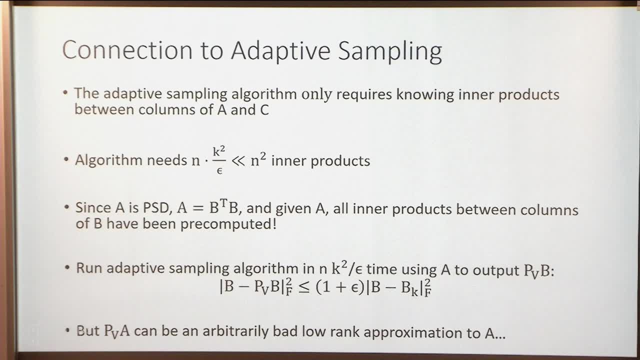 arbitrarily bad approximation to A. OK, You'd really have to crank down this epsilon to be very small as a function of the spectrum of A actually, So it doesn't quite work. But what we're going to do is we're going to, but, by the way, this is already useful. 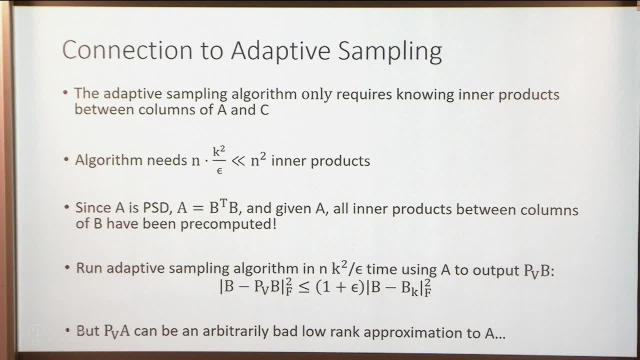 on its own, in the sense that sometimes you want a low-rank approximation to a factor of a kernel matrix And you can think of A as being a kernel matrix and this being a low-rank approximation to a factor form. But that's not what we're going to do here. 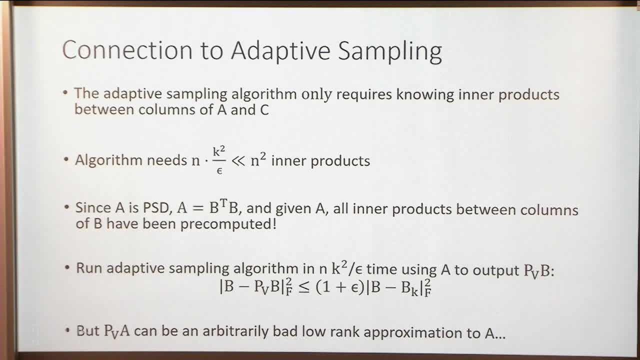 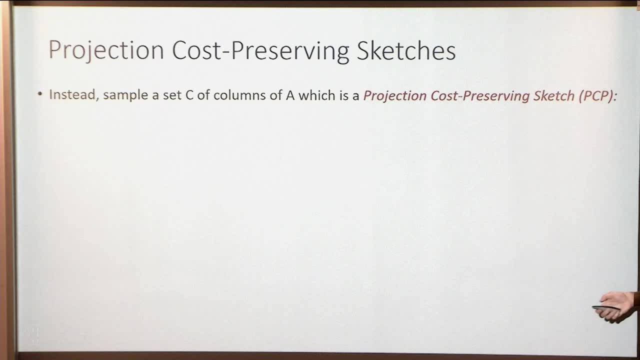 So we still want a low-rank approximation of A, And we'll see how B can still be helpful in that regard, just in a different way. OK, So what we're going to do is we're going to use the notion of what's called a projection. 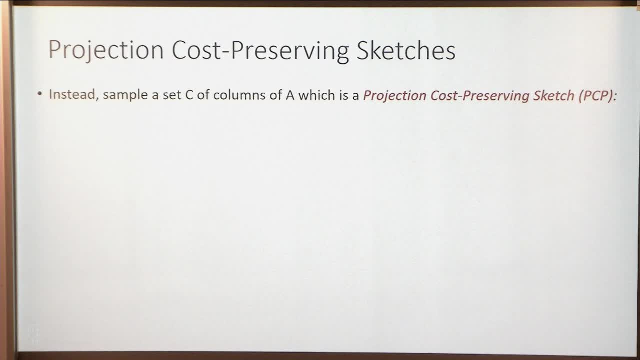 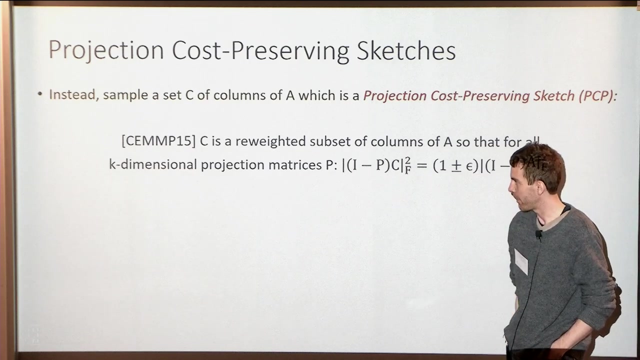 cost preserving sketch. Now this is a sample of a set C of columns of A, which has the following property: So this was, in a beautiful work of Michael Cohen et al, Very tragic news recently And what they showed is the following: that they defined the following notion: that C 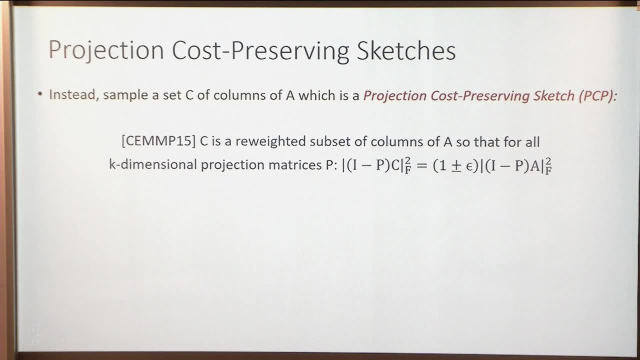 is a Is a re-weighted subset of columns of A which has the following property: It has a core set-like property, which is that, if you give me any rank, K projection matrix P, suppose I look at I minus P, the projection onto the complement of P, Suppose. 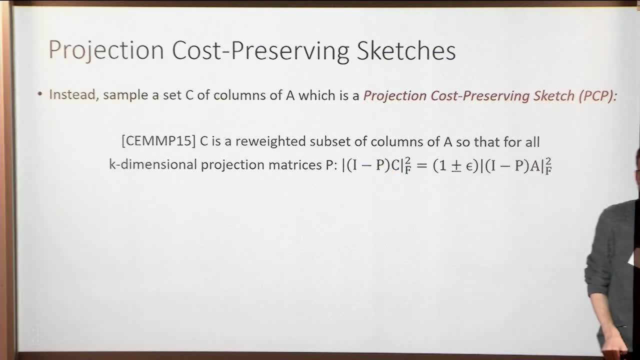 I look at the norm of I minus P times C, then that's the same as the norm of I minus P times A up to a 1 plus or minus epsilon factor. OK, So what does this mean? I have my n columns of A and I want to compute the sum of their squared distances to P. But 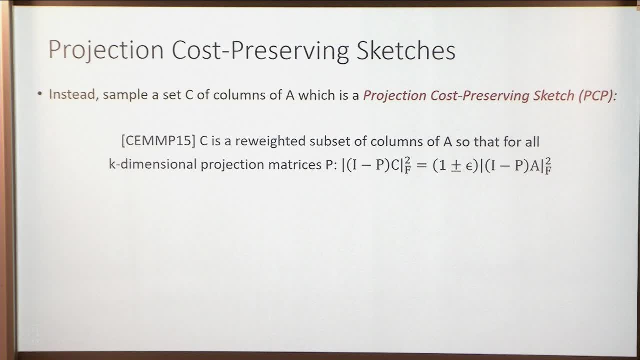 I don't want to keep A around because it's too big and it takes a lot of memory, et cetera. So I'm not going to keep it around, I'm just going to compute this C, which has a much smaller number of columns. 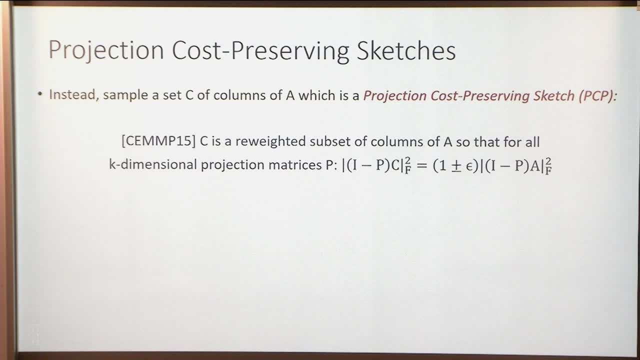 And every time you ask me what is the distance to your favorite rank K space, I'm just going to use C and compute it in terms of C And I know that's a good approximation to A. OK, So it's a core set in the sense that it holds for every matrix P. 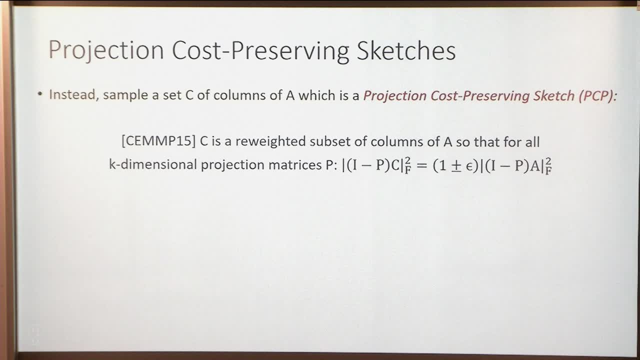 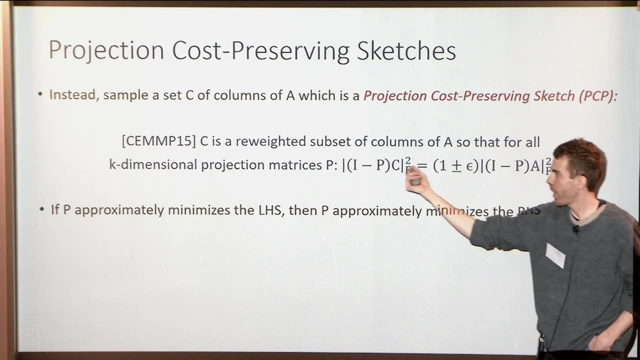 OK, OK, So it holds for every matrix P simultaneously every projection matrix P, OK. So a nice thing about projection cost-preserving sketches or PCPs, is that if you find a rank K projection matrix P which minimizes the left-hand side, it also minimizes the right-hand. 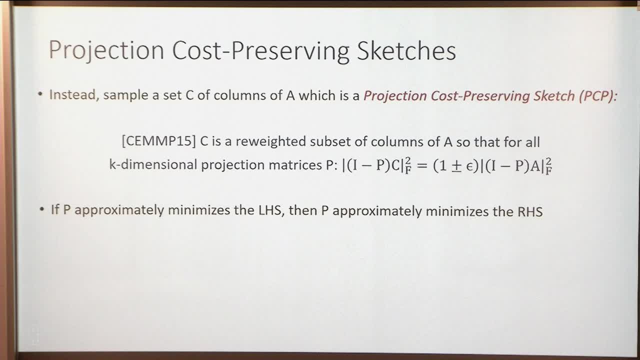 side right, Because it preserves everything up to 1 plus epsilon. So what does that mean? Well, it means that if somehow you have a rank K, projection matrix P which minimizes the left-hand side, it also minimizes the right-hand side right. 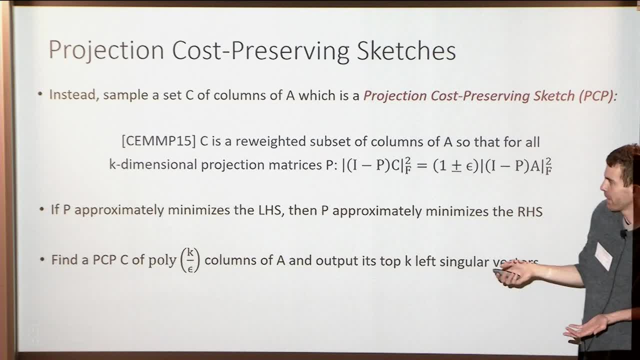 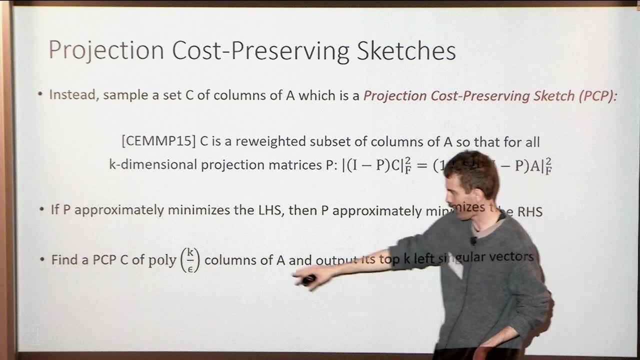 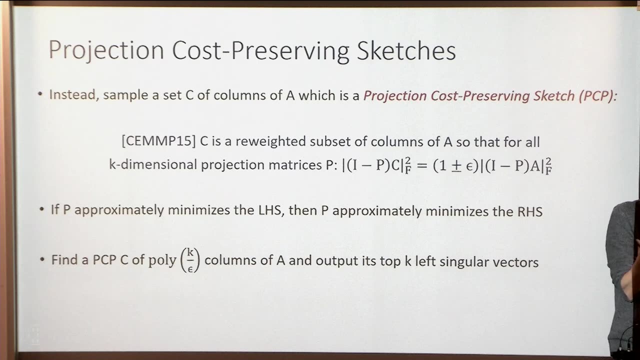 So if somehow, someway I was able to get a PCP for A, for the columns of A, with a small number of columns, say a number of columns, which is roughly like poly K over epsilon, then I could just take C and I could find its best. its top K, singular vectors, its 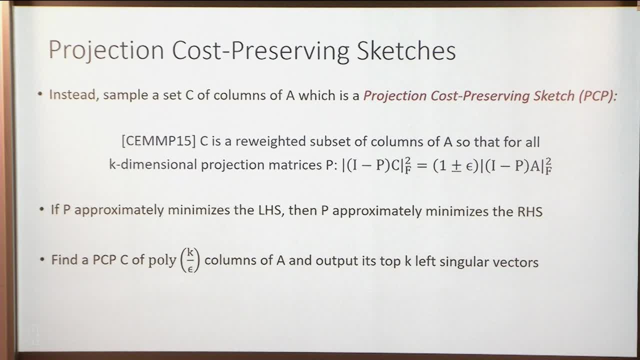 best K-dimensional space. Why? Because its best K, its top K singular vectors, minimizes the left-hand side. and so because it's a PCP, it's also, It's also a good 1 plus epsilon approximation for the right-hand side. 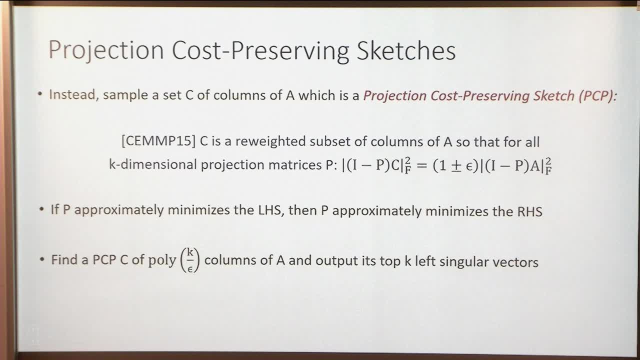 So once I have C, forget about A. I just find the top K left singular vectors of C and I get a good approximation for A. Yeah, and if C has a small number of columns I can afford to read all the entries in C. There are only N entries in each column of C and 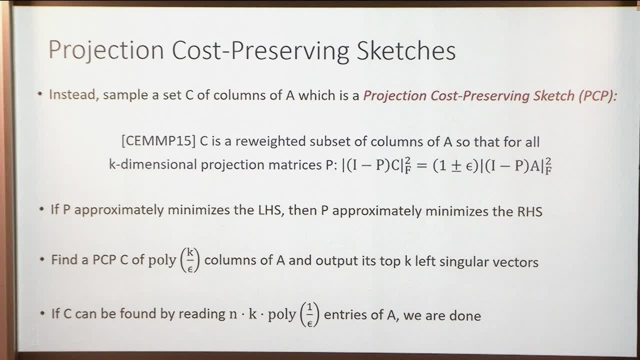 I'll get like roughly N poly K over epsilon time. So really, if we can find this PCP C, Yeah Yeah, Yeah Yeah, Also in sublinear time, like roughly N time, then we're done. Our goal is just to find this PCP. 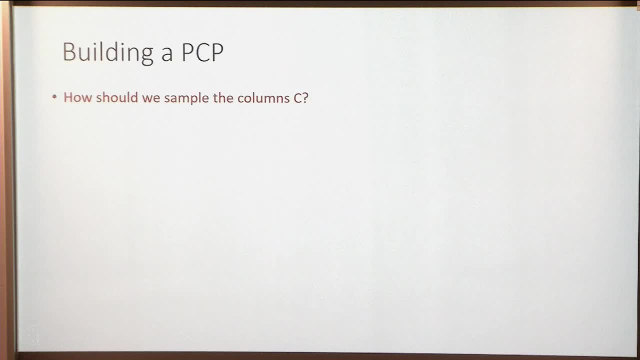 Okay, Yeah, So how are we going to do that? So we want to sample columns of A to build a PCP. So we're going to use a notion called the ridge leverage scores, and it's not For this talk, it's not so important if you understand their definition. 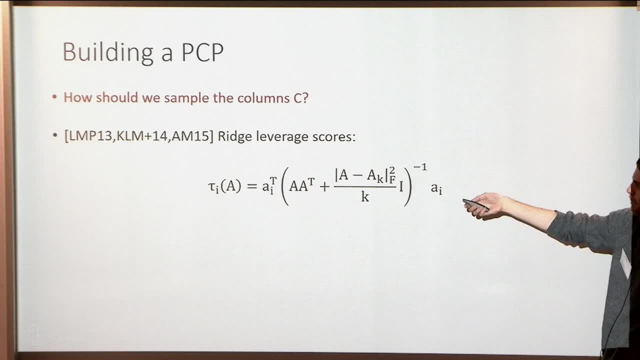 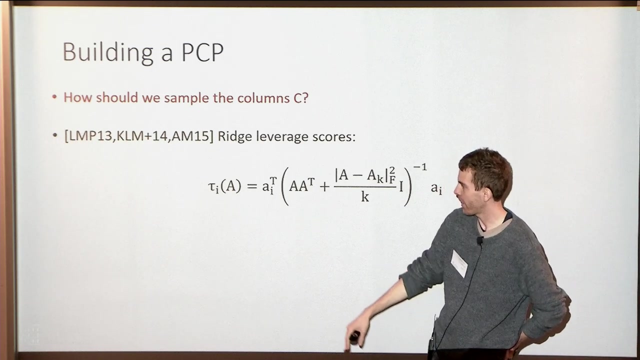 But this was introduced in several different works at the same time, similar times: Lee Miller, Pang, Kapilov et al Alawi and Mahoney. Basically these are. So there's just some quantity for each column of A. I define what's called a ridge leverage. 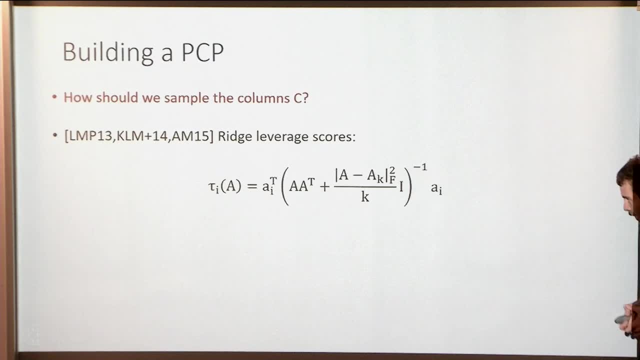 score tau sub i of A. What this quantity is is. it gives a smooth version, Okay, Of the standard rank K leverage scores. if you've seen these before, So yeah, if you haven't seen these before, it's really not important what they are for. 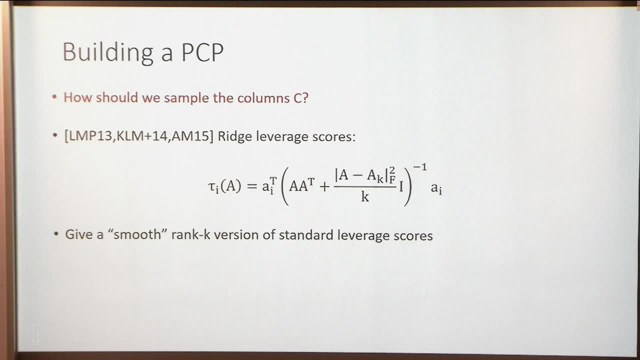 the talk, But the rank K leverage scores. what they are is, if you take the top K left singular vectors of a matrix, these top K left singular vectors, they, If I take the top K left singular vectors of a matrix, U sub K, then I know the squared. 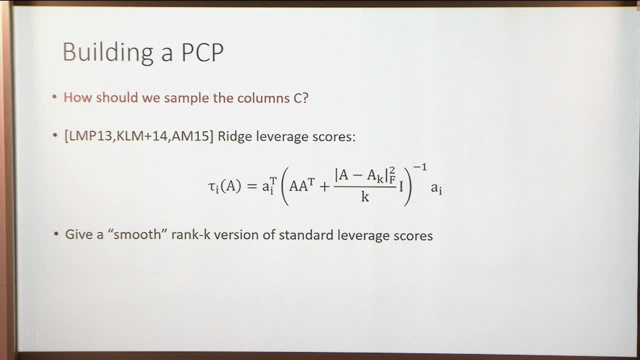 column norms of this matrix. The matrix are all one because these are orthonormal vectors, And the squared row norms, the i-th squared row norm, is called the i-th leverage score, the i-th rank K leverage score. Okay, And these can be arbitrary. 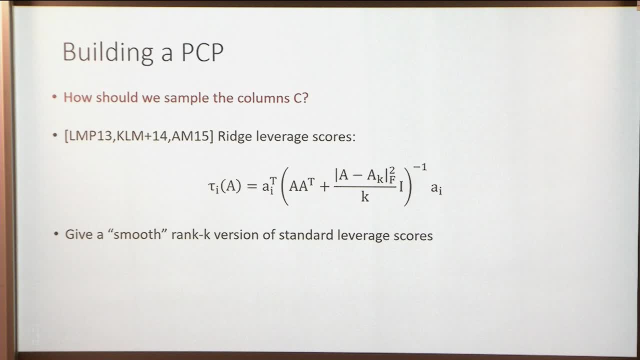 I mean they sum up to K, since the sum of the columns is K, the sum of the rows is also K. But in any case, the ridge leverage scores. they're useful as they give sort of a smoother version of this. 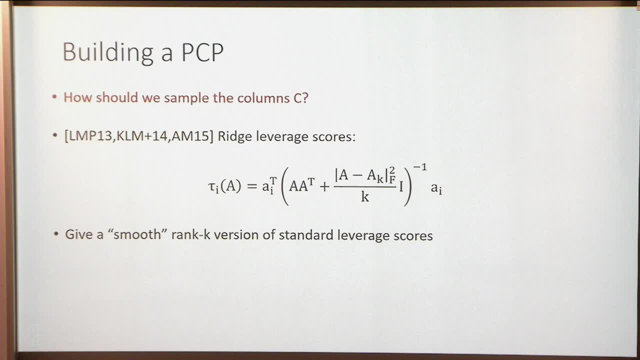 I mean they're robust to Slight perturbations in A et cetera. The sum of all the rank K, all the ridge leverage scores, is at most 2K, so slightly larger than K as it is here. 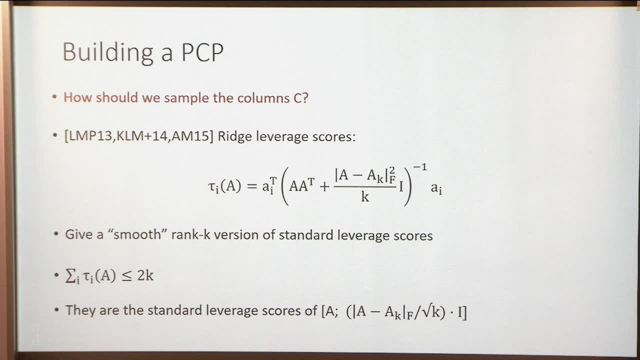 But it's still small, which is what we'll need for sampling-based algorithms. And there's some connection to ridge regression, if you've seen it before. These correspond to the standard leverage scores of taking your matrix A and concatenating them with a scaled identity matrix. 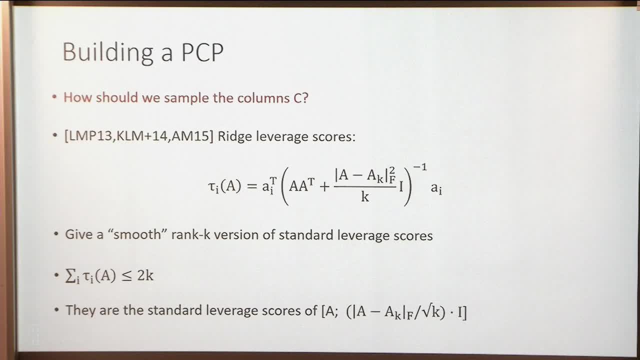 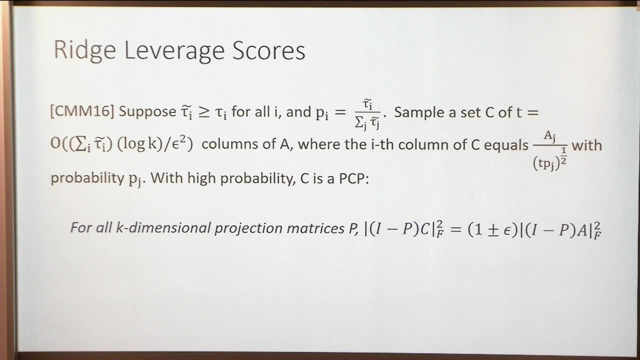 But again, it's not so important if you haven't seen it. So how are we going to use the ridge leverage scores? So it turns out that they provide a PCP. Okay, So let me say that more precisely. So, in work of Cohen, Musco and Musco, they showed the following: 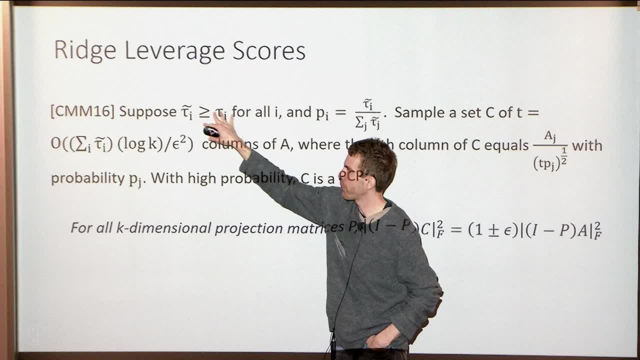 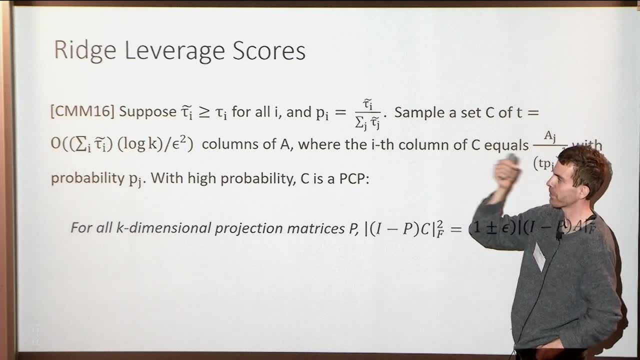 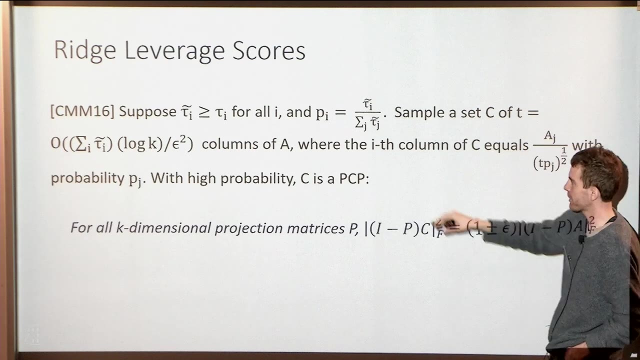 Suppose you have overestimates- tilde tau i for each of your actual ridge leverage scores. tau i, Let's define a probability distribution on the columns of A. p sub i corresponds to the probability for the ith column And it's just proportional to tilde tau of i, the ith approximate ridge leverage score. 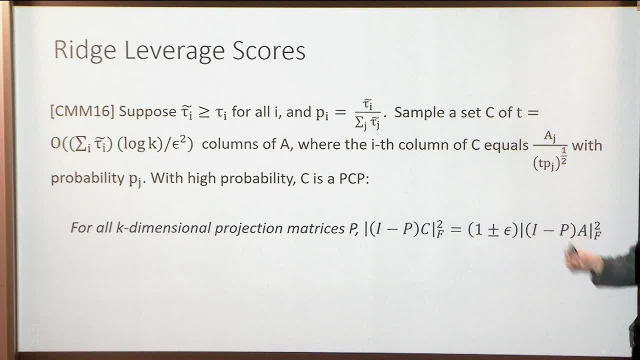 Then we're going to sample a set C of T columns of A- Ignore for the moment what T is, But we're going to do it with replacement And the ith column of C is just going to equal the jth column of A with probability. 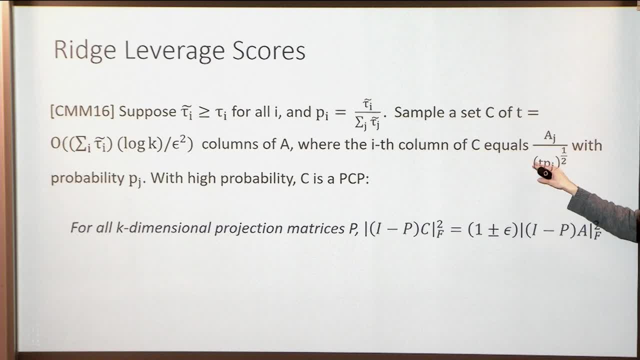 p sub j, scaled by roughly square root of T times the probability that we sample that column. Okay, So we're sampling T columns. We scale by roughly 1 over the square root of T times the probability that we sample it. Okay. 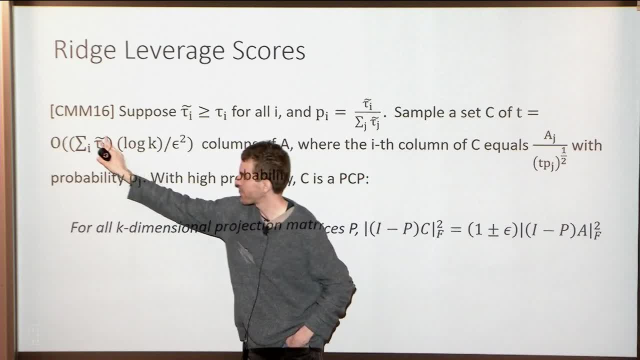 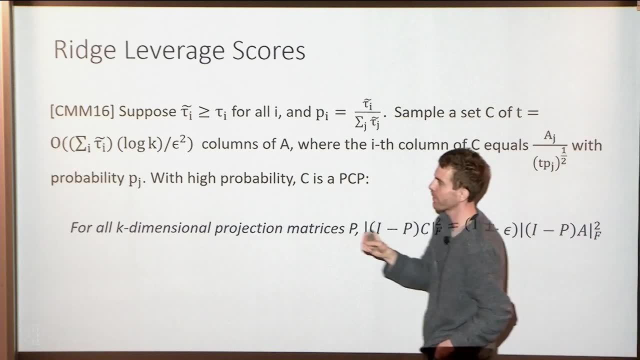 The number of columns you sample. it's proportional to the sum of your overestimates. The sum of your overestimates to the actual ridge leverage scores. Okay, So if you had the actual ridge leverage scores, the sum of them would be k. 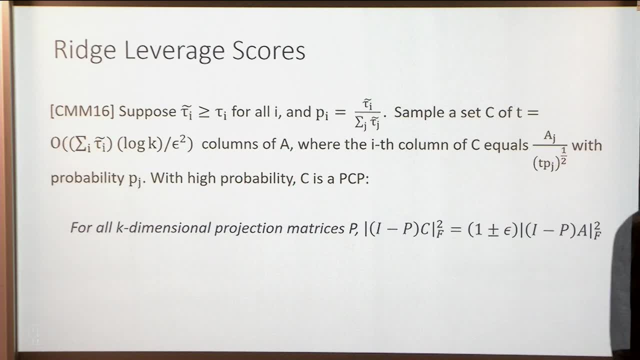 And you would sample roughly k log k over epsilon squared columns And yeah, if you have sort of crude estimates you have to sample more. But they show that if you sample according to this distribution you get a PCP. And we said if you have a PCP then we're done with our problem. 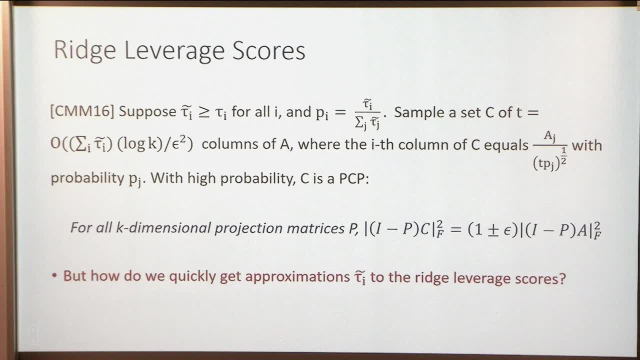 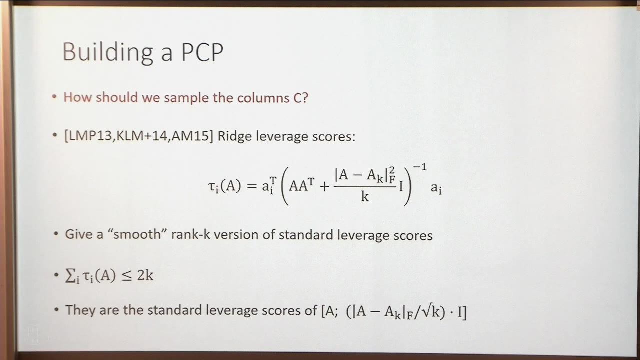 Okay, But the question is: you know how do we get the ridge leverage scores, or how do we get good approximations to them in sublinear time, Okay? So I mean, it doesn't seem obvious how to? The ridge leverage scores are defined by some complicated expression. 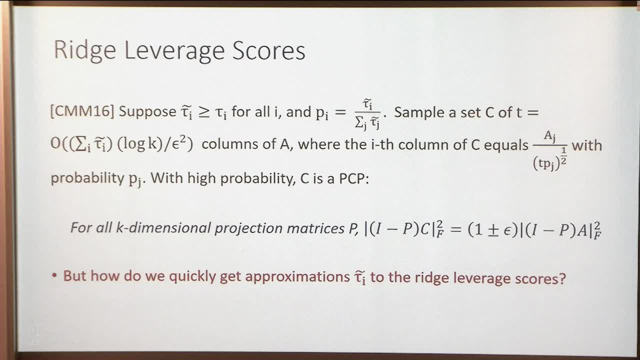 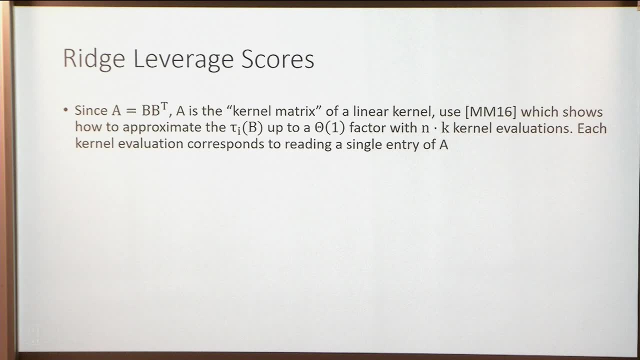 How can we get these in sublinear time? So what we're going to do is use the connection that I mentioned earlier to this literature on kernel matrices In machine learning. So we said A is equal to B, B transpose, since it's PSD. 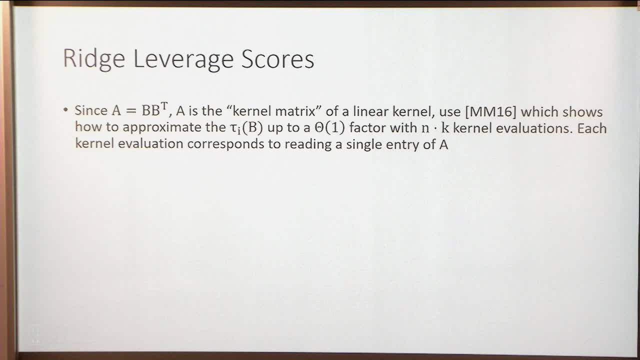 So we can think of A as being the kernel matrix of what's called the linear kernel. And there is work by Musco, and Musco in last year, which shows how to approximate the ridge leverage scores of B up to a constant factor. And the time that you need is 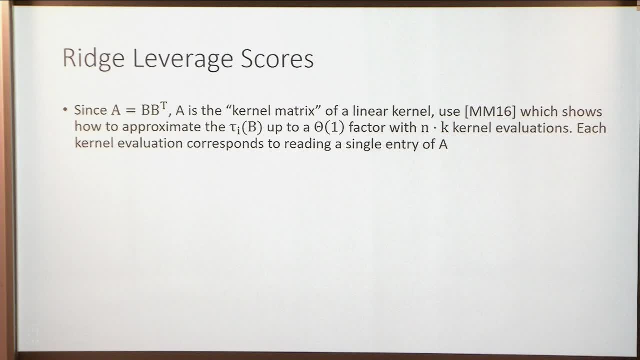 Okay, N times K kernel evaluations, And now we're going to use this connection again that one kernel evaluation is just an entry of A Right, Because this is a dot product. A kernel evaluation for a linear kernel means a dot product. So there's an algorithm that can compute the ridge leverage scores of B each up to a constant. 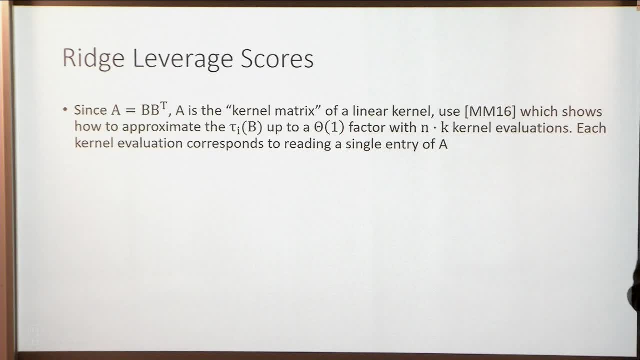 factor by reading only NK entries of A. Okay, Okay, And what we show is that the ridge leverage scores of A are related to the ridge leverage scores of B. Okay, Even though we said: if you get a good low-rank approximation to B, it could be arbitrarily. 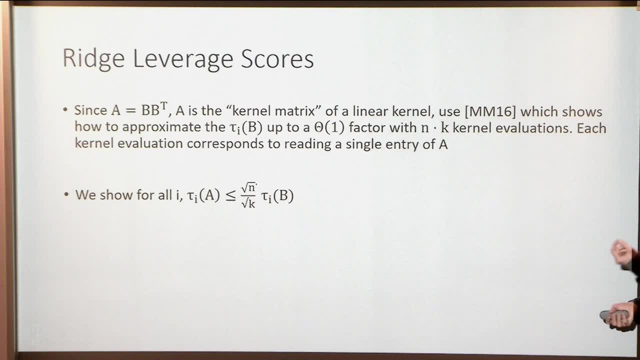 bad low-rank approximation to A, But what we do have is that at least the ridge leverage scores of B, if we scale them by roughly root N, then they're overestimates to the ridge leverage scores of A. Okay And okay. so what is the sum of all of our overestimates? 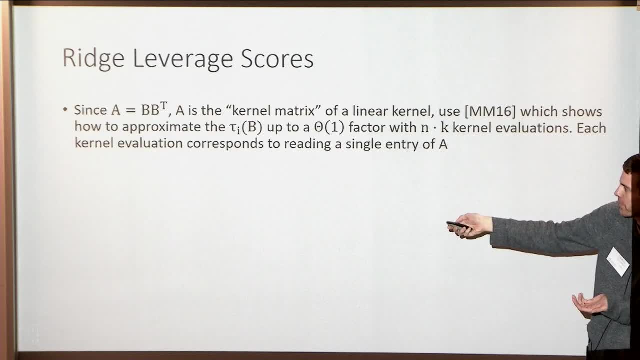 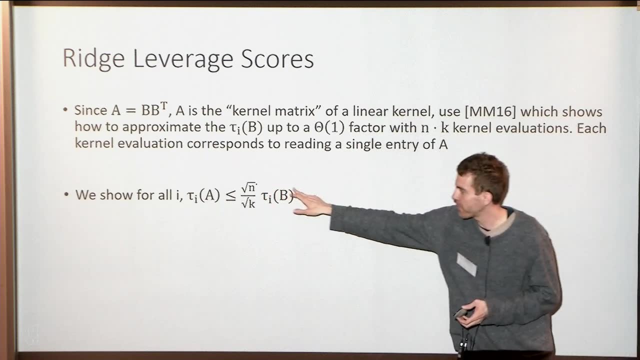 This is the. this is the tilde tau i we're going to use. It's going to be root N over root K times the ridge leverage score of B. Well, we said the sum of all the ridge leverage scores of a matrix is roughly K And the number of columns 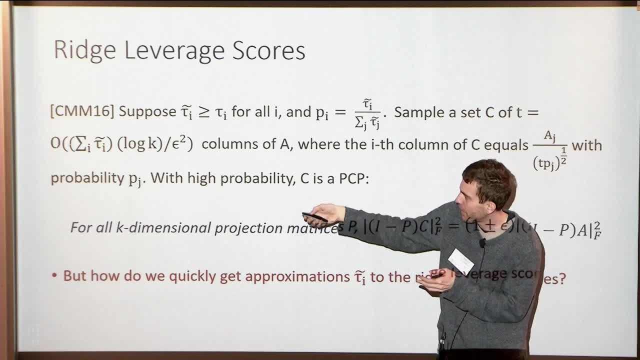 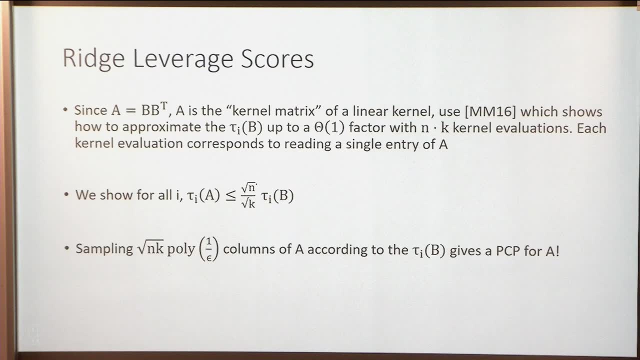 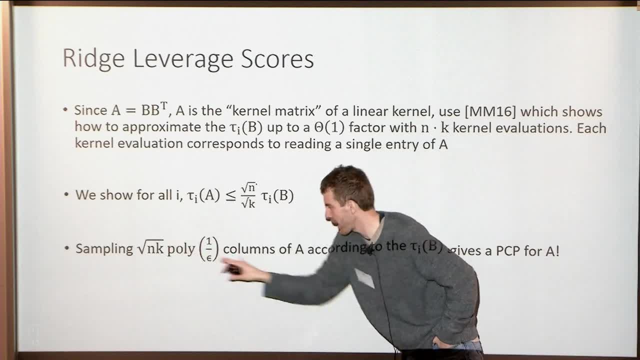 It turns out that if you sample roughly root N, root K columns of A according to the ridge leverage scores of B, then you get a PCP for A. Okay, And this PCP. so so this, this, this already gives us an algorithm. 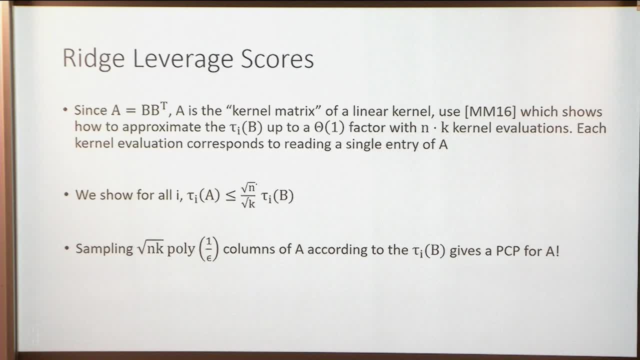 We know in order N time we can find all these good approximations to the ridge leverage scores of B. Then we know that if we oversample by a root N factor, if we sample roughly root N K columns of A proportional to these, then we'll get a subset of root N columns which is a PCP. 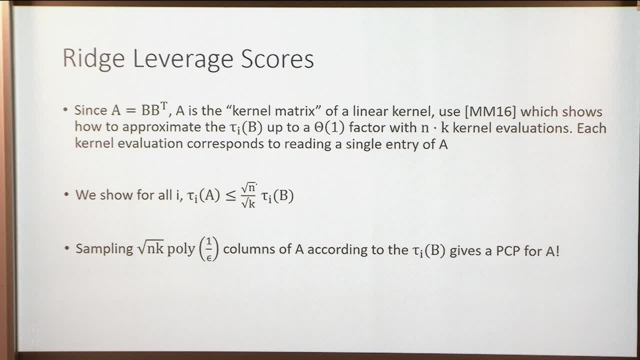 for A And therefore we can just find the best rank K approximation inside of there. That already leads to an N, to the three halves time algorithm, which is already, you know, sublinear time for certain values of N and Z of A. The final step which we really want. 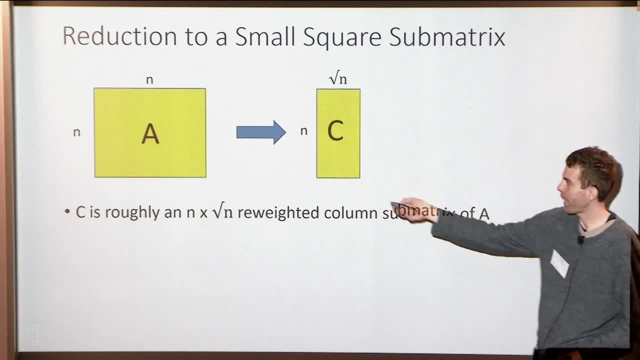 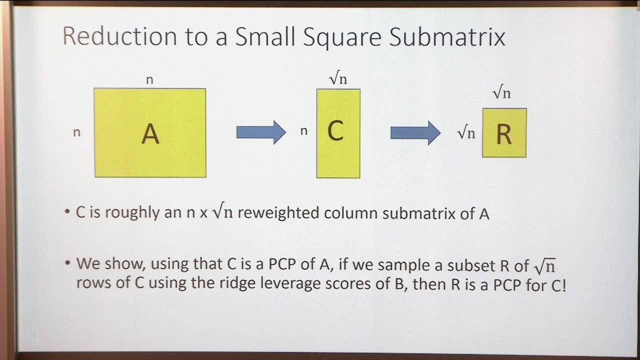 is actually an N time algorithm. What we've shown is how to take A sample roughly root N columns to get this matrix C. Um, there's one other step is we show how to sample roughly root N rows of this matrix C to get a matrix R, which is root N by root N And it. it turns out that actually the 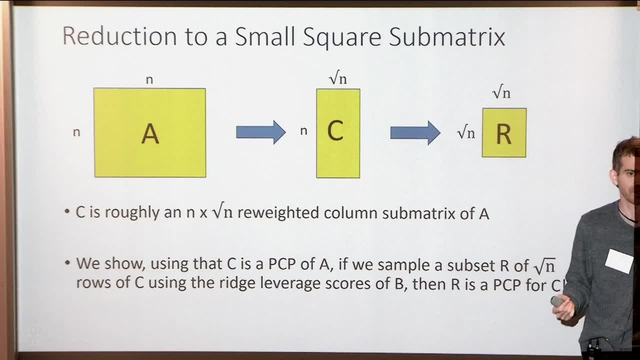 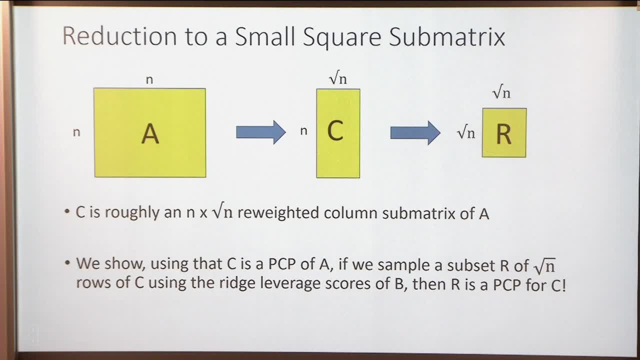 of that Um, but the but. but the point now is: R is a very small matrix: root N by root N, And now you can do whatever you want on this. Okay, So you can afford to run these input sparsity time algorithms on R, because they'll take 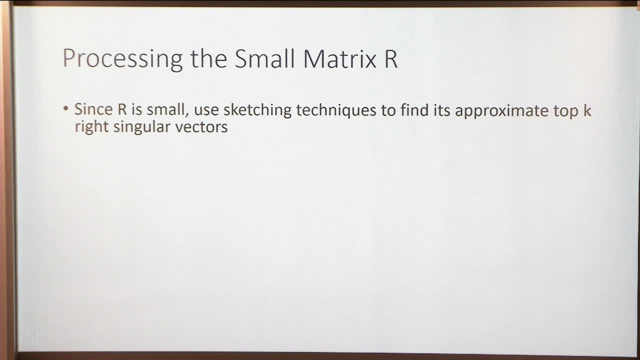 it most N time. Okay, So since R is so small, you can use the earlier sketching techniques I described to find its top K-right singular vectors. Since R is a PCP for C, its top k right singular vectors can be used to find the top k left singular vectors of C. 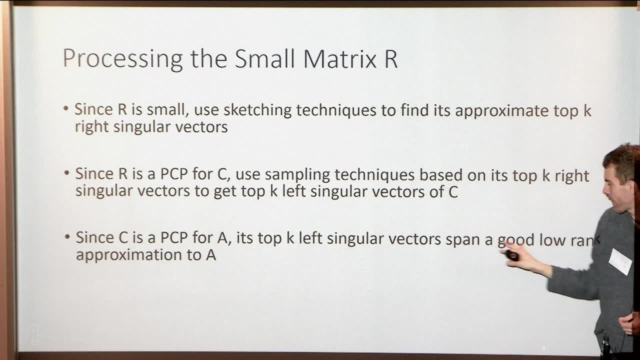 And since C is a PCP for A, its top k left singular vectors are a good low-rank approximation to A. So that's the overall logic behind the algorithm. You reduce it to a small square matrix. do whatever you want. find the top k singular vectors. 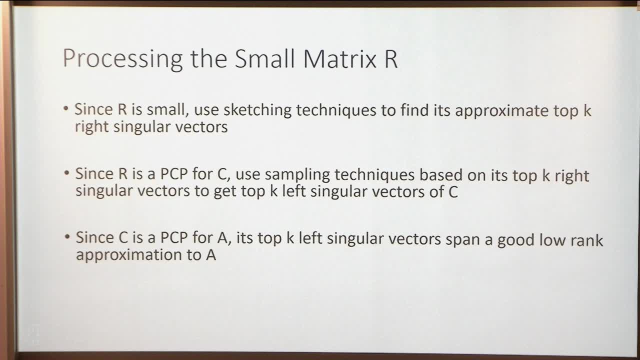 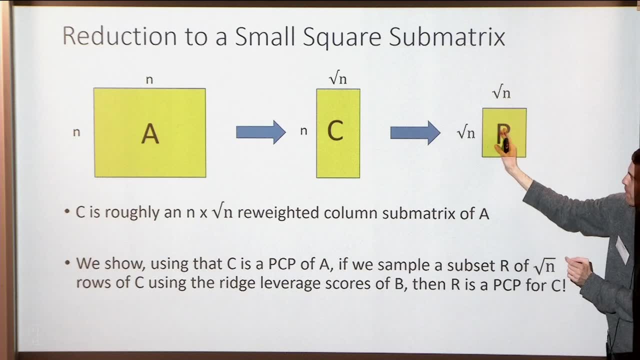 Then there's a procedure of using those top k singular vectors to find the k, because R sits inside of C here, So I find its top k directions and I can actually sample from them to get k directions inside of C that are very good for C. And since those 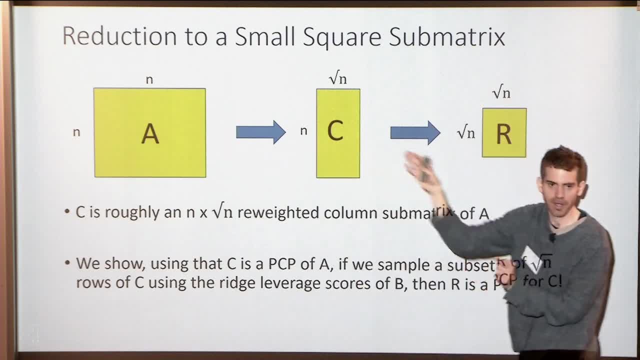 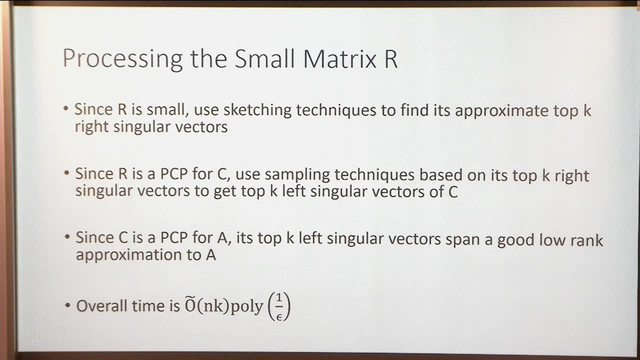 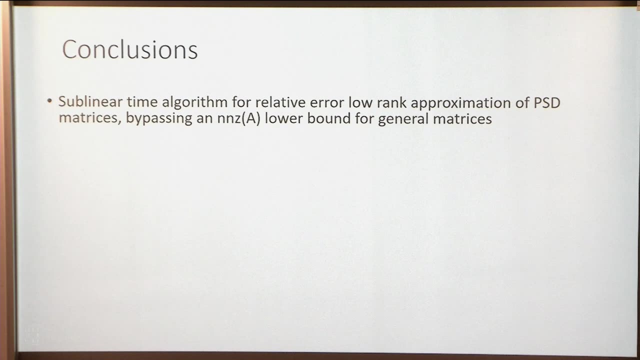 are very good for C. they're also very good for A because C is a good representation of A. It's a PCP of A. So overall the algorithm runs in nk poly 1 over epsilon time. So just to conclude, we give the first sublinear time algorithm. 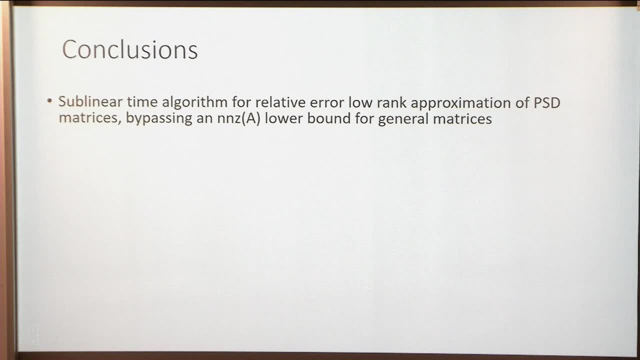 achieving relative error, Low-rank approximation for a natural family of matrices. so for PSC matrices, which bypasses this n? nz of A time lower bound for general matrices, In fact, our concrete bounds are fairly tight. I mean we're getting n times k entries. 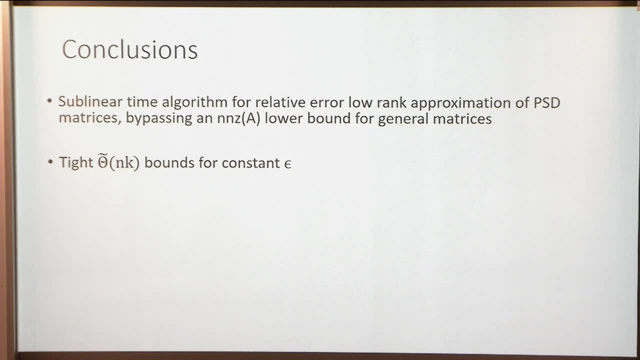 and we can prove a lower bound for that. You might ask for other error measures. Not everyone is just interested in the Frobenius norm. It turns out that if you want spectral norm error, that's impossible In sublinear time. we can show that. 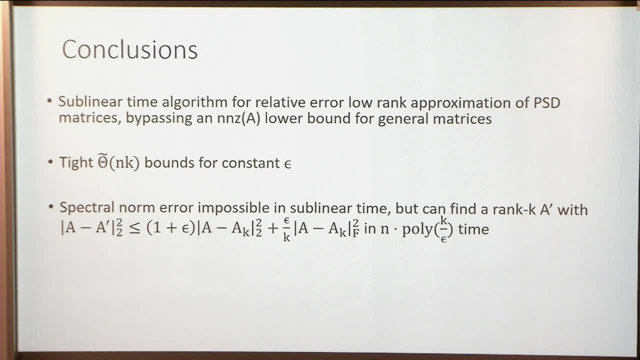 But you can get sort of a mixed guarantee where it's like a mixture of a spectral and a Frobenius guarantee. You output a rank k matrix, A prime for which the squared spectral norm difference is at most 1 plus epsilon times the optimal squared spectral norm. 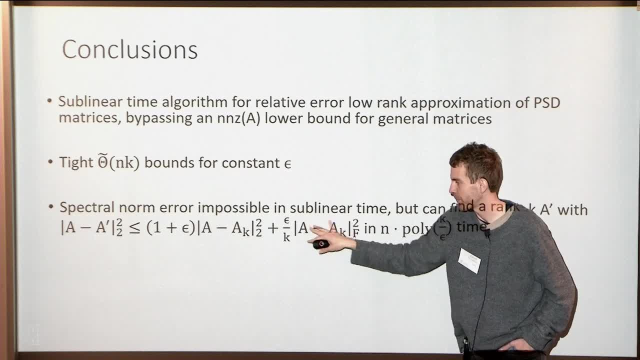 difference plus a term that depends on the Frobenius norm. So epsilon over k times the squared Frobenius norm of a tail That you can do in sublinear time. I mentioned this earlier problem in the talk of. sometimes you want to output a matrix which is itself PSD. 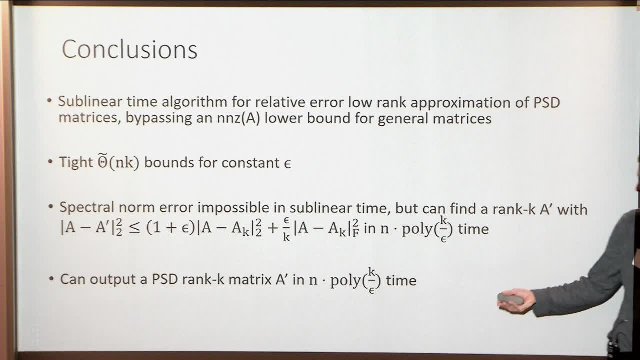 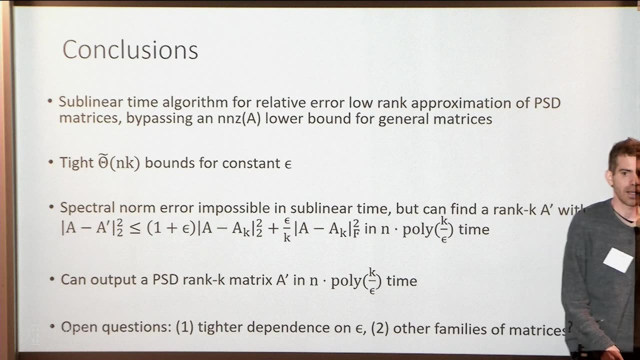 You want your low rank matrix to be PSD. We can do that here too. So we're given a PSD matrix and we output a rank k PSD matrix in roughly n time. And the open questions here? so a natural question is to get tight bounds on this epsilon parameter. 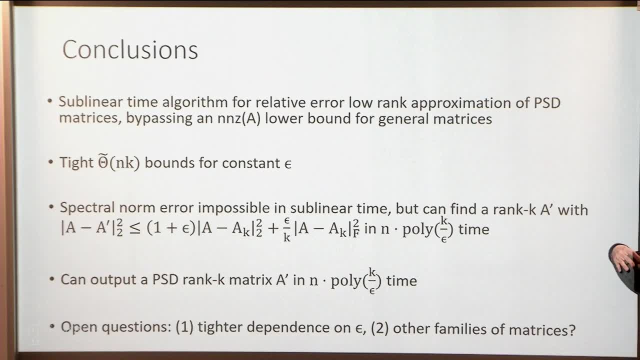 Our upper bound is roughly like 1 over epsilon to the 2.5.. and our lower bound is roughly one over epsilon And sort of more generally like: are there other natural families of matrices for which you can bypass, you know, skirt around this N and Z of A time lower bound. 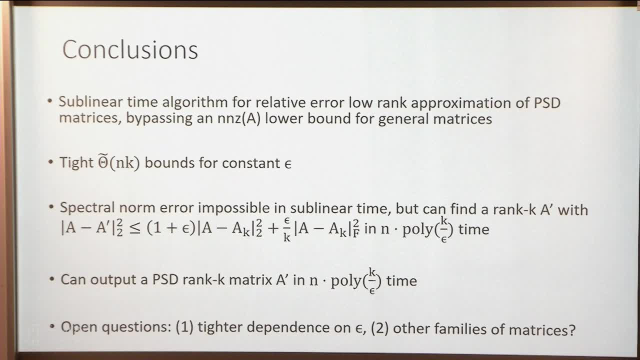 and get like a truly sublinear time algorithm. So that's all, Thanks. Slightly behind schedule, maybe, one quick question: What if the matrix is just a little bit indefinite? So you know, if I do round off there, it's not quite PSD. 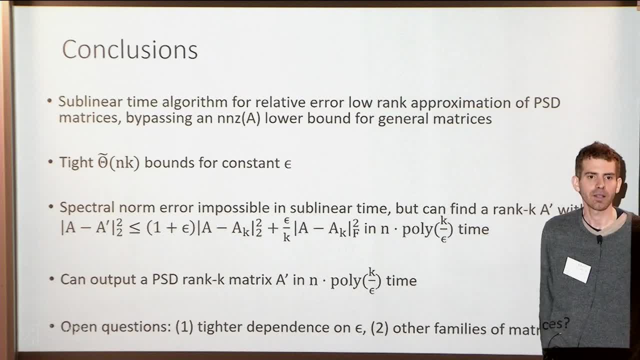 I see. so you have like your PSD matrix plus an error matrix Plus an error. yeah, If it's small enough and if you just get a in certain cases, if you could just get a low-rank approximation to the PSD part. 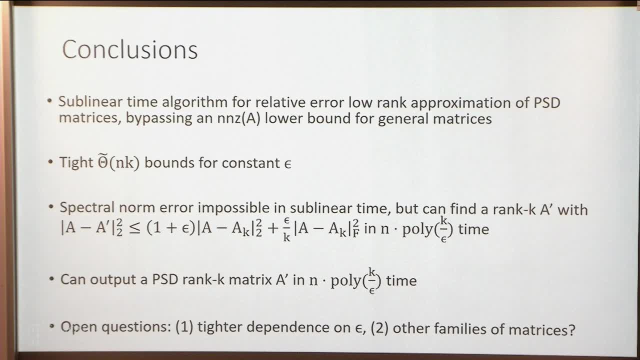 Yeah, Use these techniques. Use these techniques. I'm not sure how robust it would be in that case. Like, certainly, if the error is small enough, then I think this should go through, but I don't know exactly what the limit of that is. 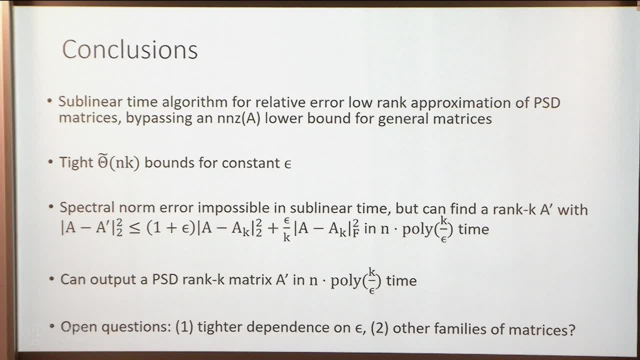 Yeah, Good question. yeah, Okay, All right, thank you. So, while the next speaker is setting up, I just wanted to make a final announcement regarding the